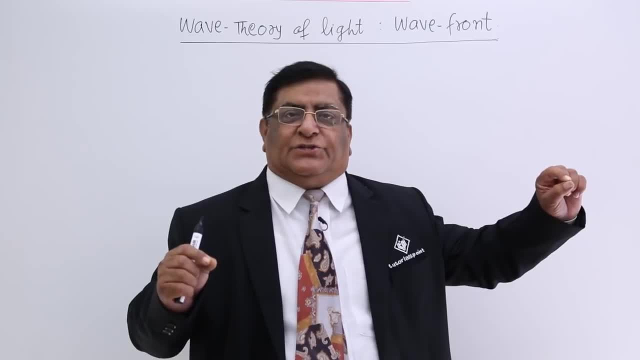 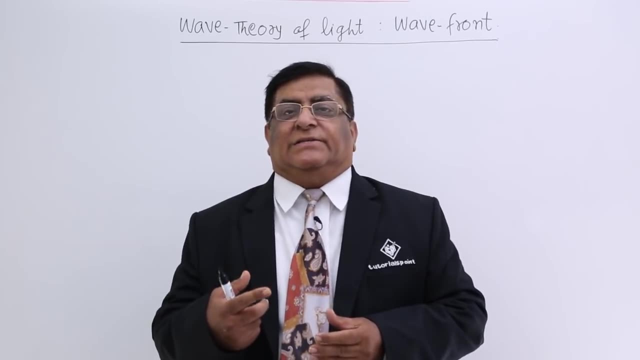 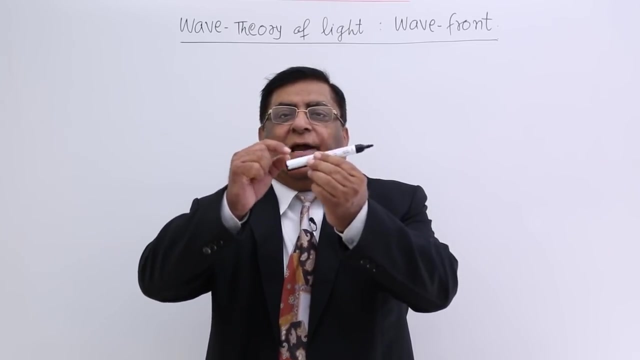 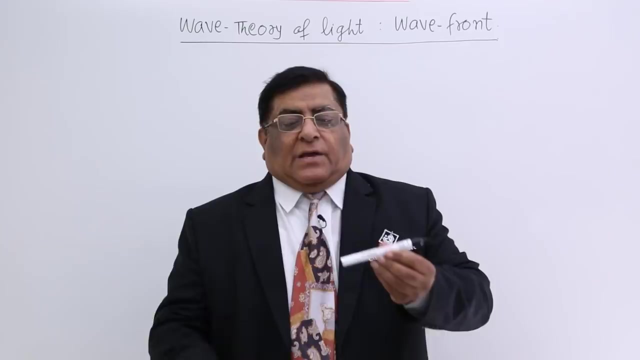 from one location reach another location, how it does In the material medium. we used to understand the things like a rope in a rope. we vibrate this portion and this portion will also vibrate because there is a connection between the two And this disturbance goes. 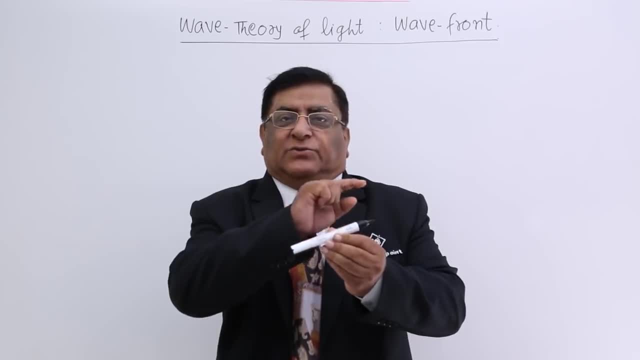 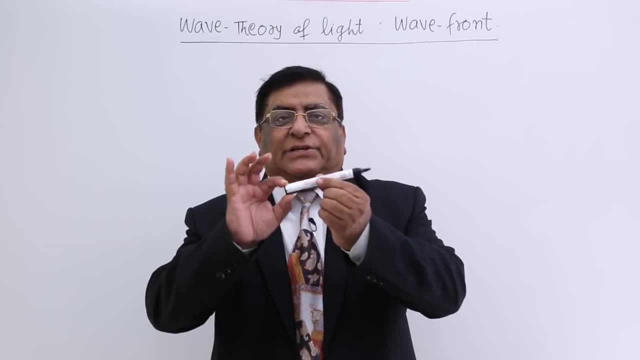 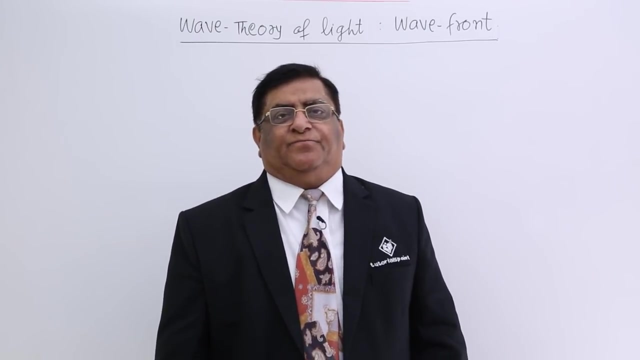 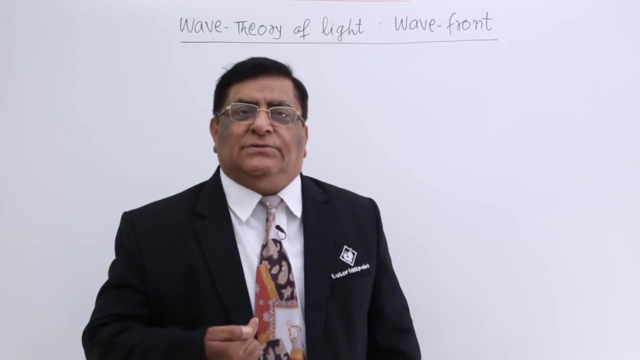 here. this disturbance goes here, This goes here, this goes here and this way. this was one method. that is how energy used to go from one place to the other place. that is, disturbance goes from one place to the other place. Another method, very popular method of sending energy was to shoot a bullet When 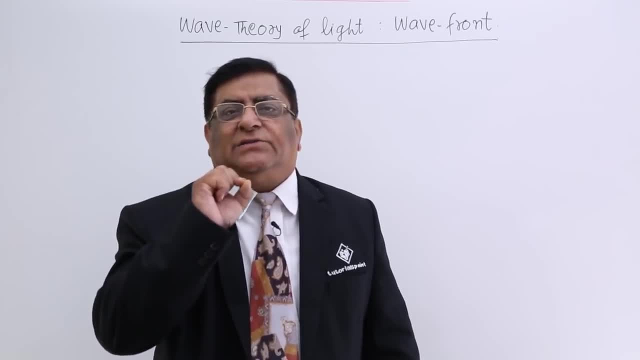 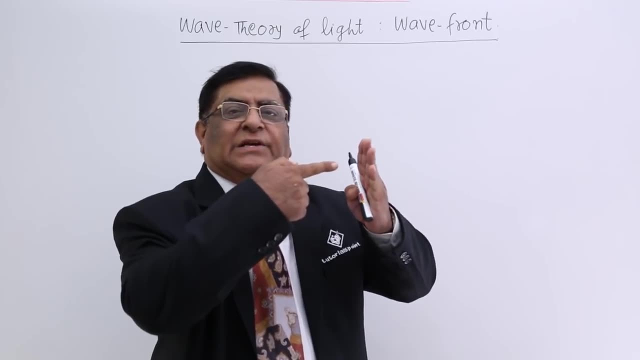 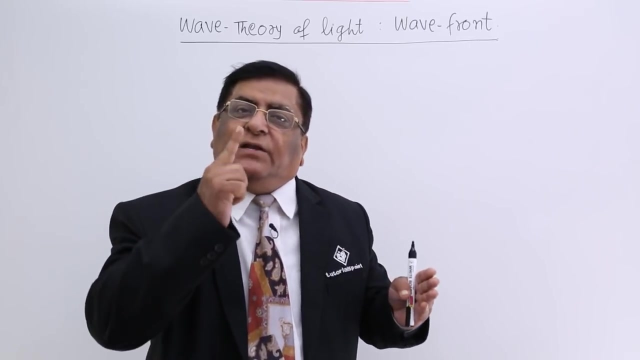 we shoot a bullet. a bullet has got mass, it has got velocity, it has got kinetic energy And it goes there and the moment it touches the target it stops and all that energy is transferred here. So the energy has moved along with the bullet. that is the method. how? 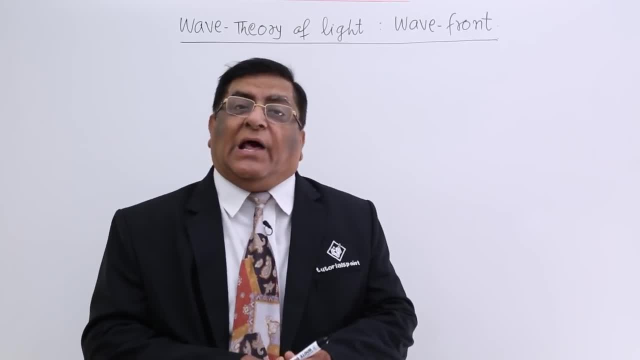 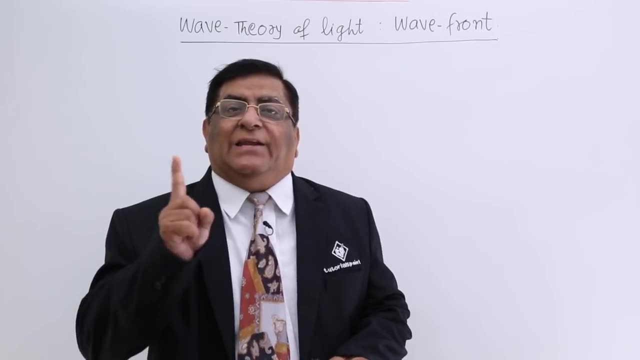 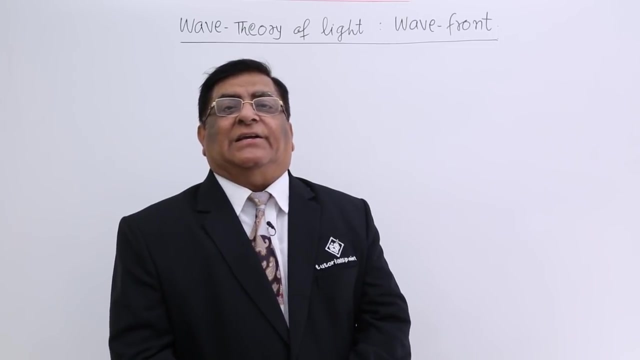 matter takes the energy. but how light takes the energy. it depends upon the effect: whether we treat light of carrying energy as material carrying carries or we take it as the energy comes from sun. light comes from sun Because we were very much acquainted with the methods of material carrying the energy. 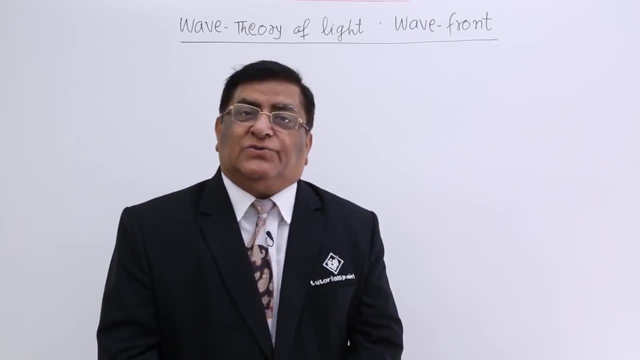 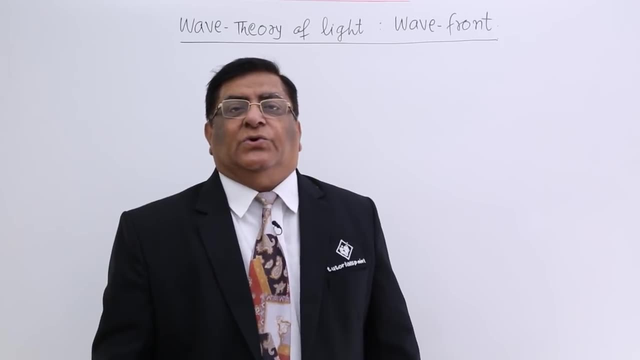 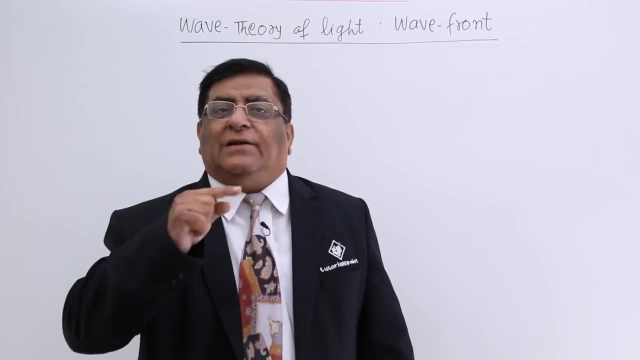 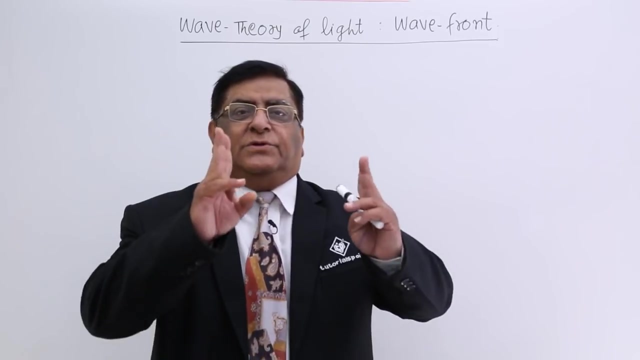 we were thinking that the light is also carrying energy in the same manner, that is, in the straight line. So Newton made this theory that light travels like a bullet and it travels in a straight line. and there was a very famous experiment by Newton's where he put three holes in one. 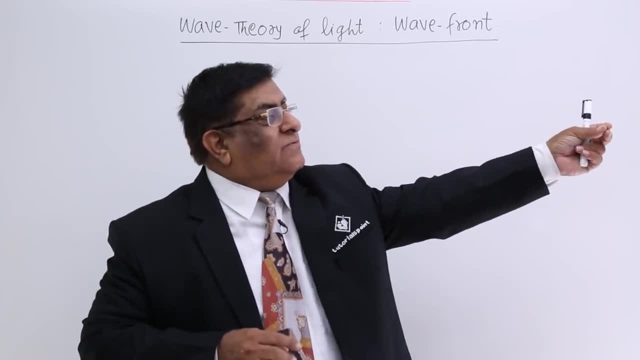 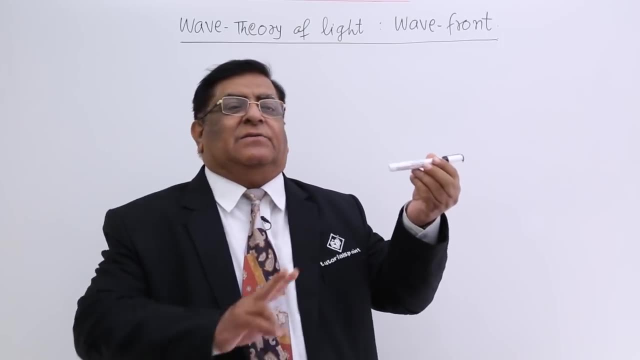 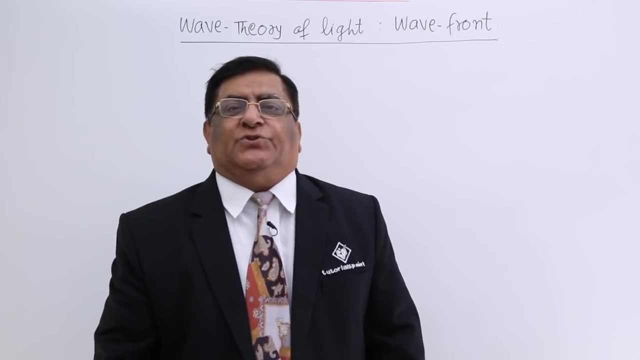 line and see through it. So the light was visible through the three holes. because three holes were in one line, He disturbed the lines by displacing any one hole, So And then the light was not coming. so it was simple enough to show that light travels in. 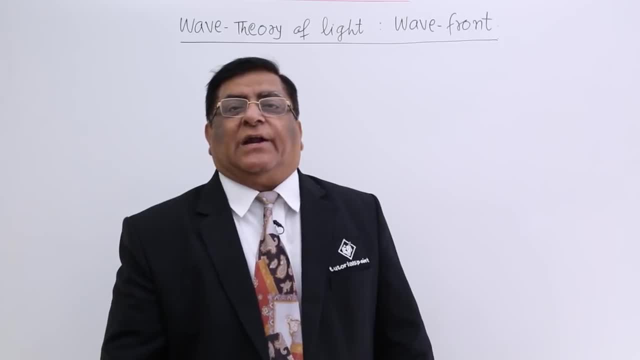 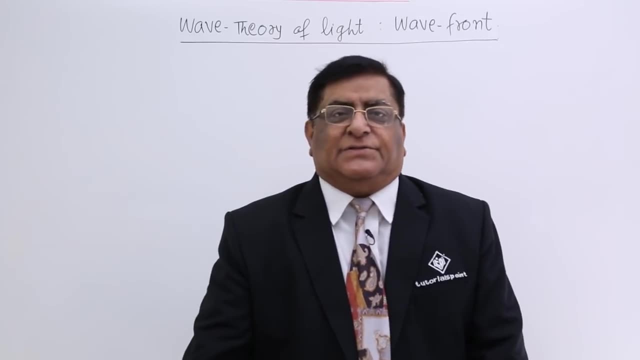 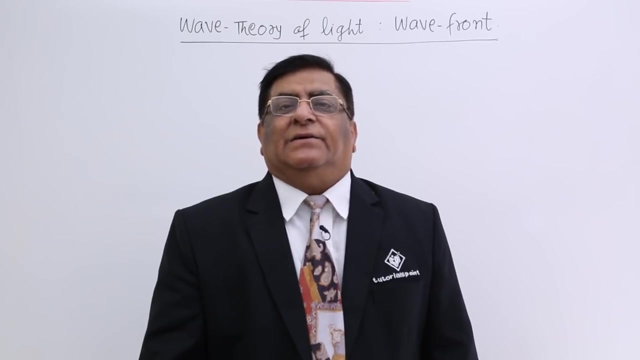 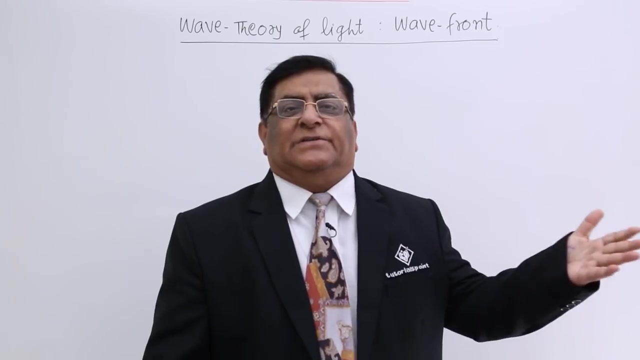 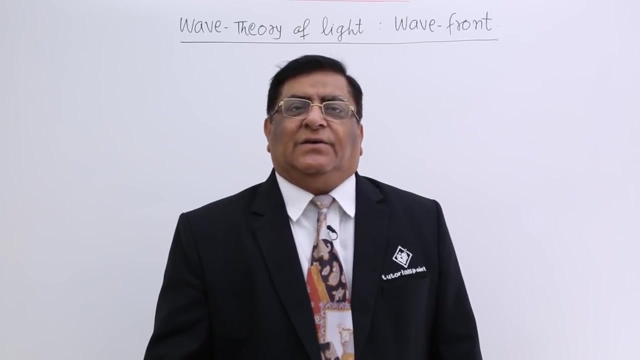 a straight line and it cannot travel without a straight line. But later there were different theories and one theory was put forward by Huygens and it was again reinforced by Fresnel And many of his disciples, Youngs and other scientists. what was that theory? 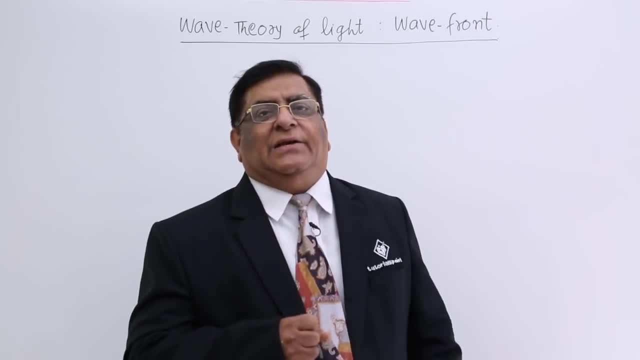 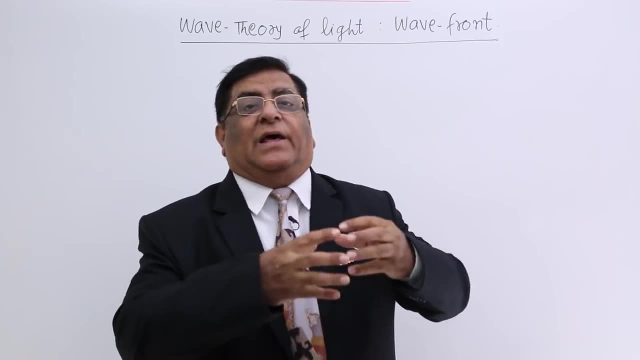 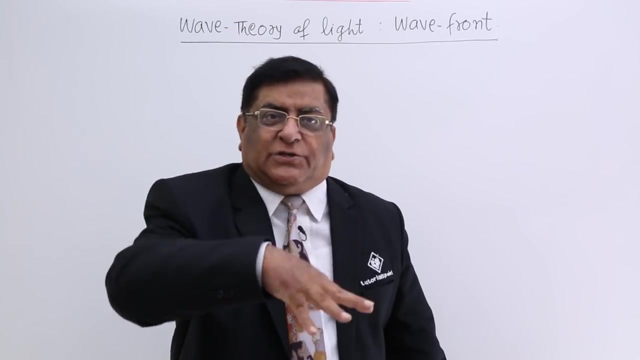 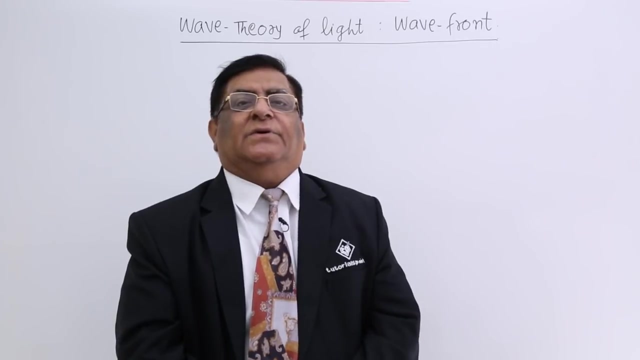 They say that the light is energy and it spreads. it spreads like water spreads all around it. If we fill water at a place, or if we put a stone in the water, then what happens? we see the waves and the disturbance of water created by the stone. disturbance is a energy. 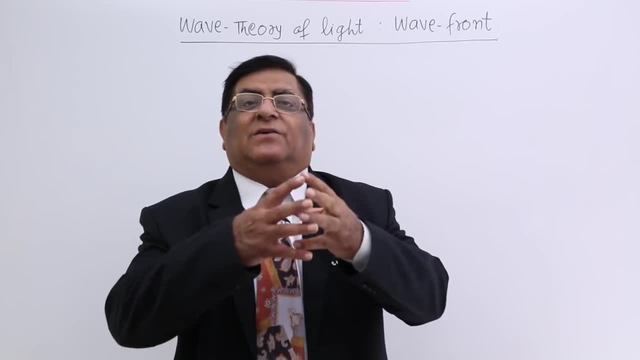 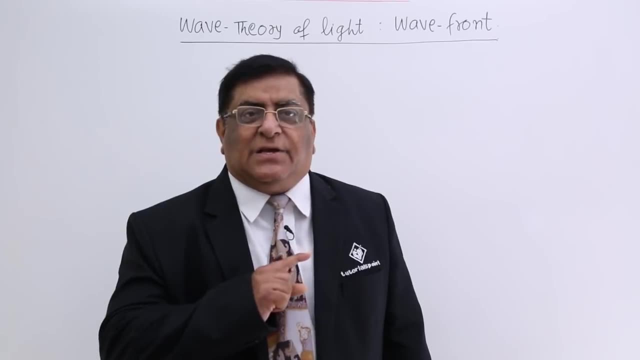 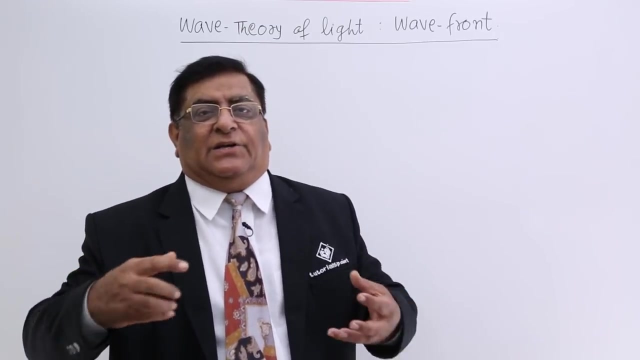 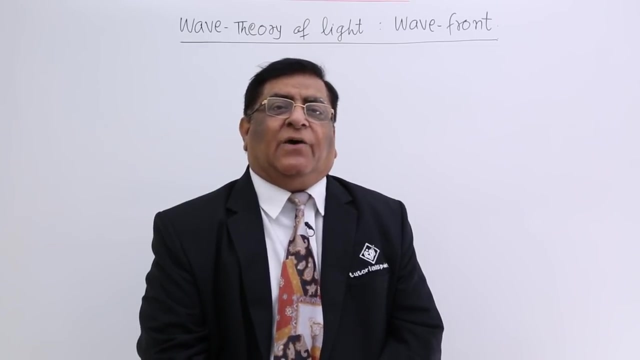 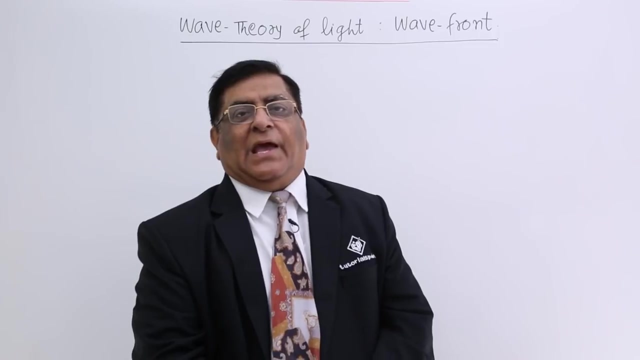 and that disturbance spreads all over. So that is also energy, that is also disturbance and that also moves, because it is in all the direction. We do not say it is one direction, It propagates in all the directions. Ok, So they say, like we have waves in the water, similarly we have waves in the light. 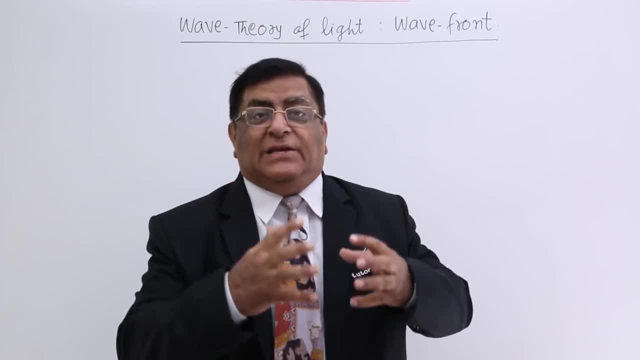 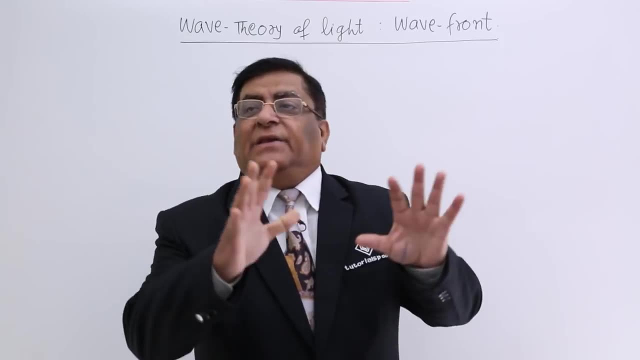 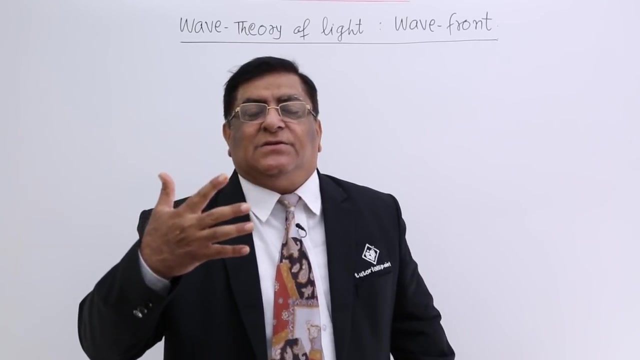 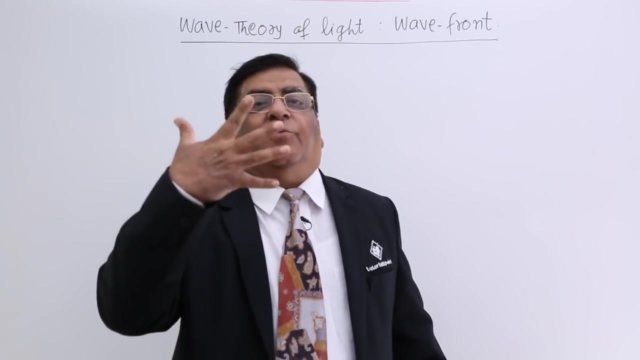 And this waves in a medium, and the waves in the medium gives us a sensation of light. Medium is everywhere, but when there is a disturbance, a wave comes, a wave comes, a wave comes. then we feel the sensation and we say that we are observing the light. 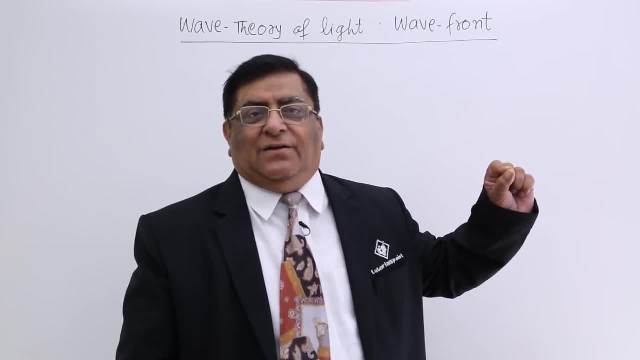 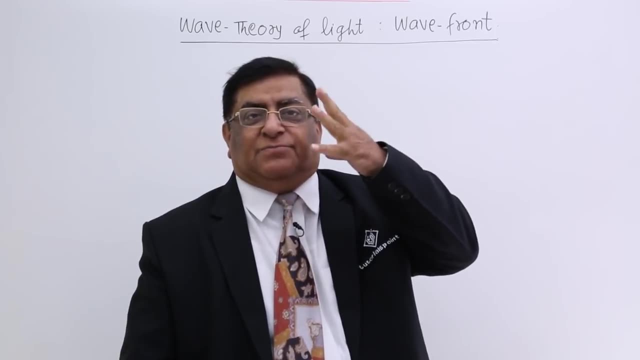 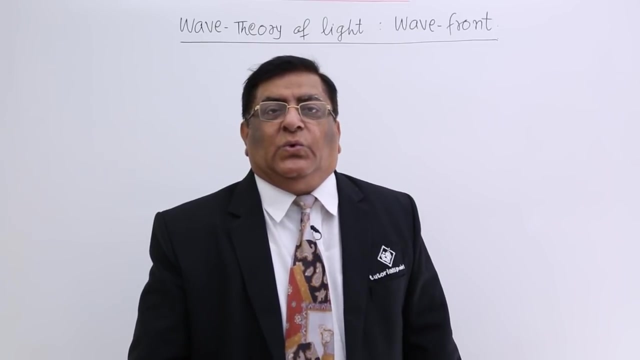 So at one place we lighten a candle. From here, the disturbance start in the form of waves. Those waves reach my eyes. there is a sensation, and I am able to see the candle. So then they were supposed to tell us Ok. 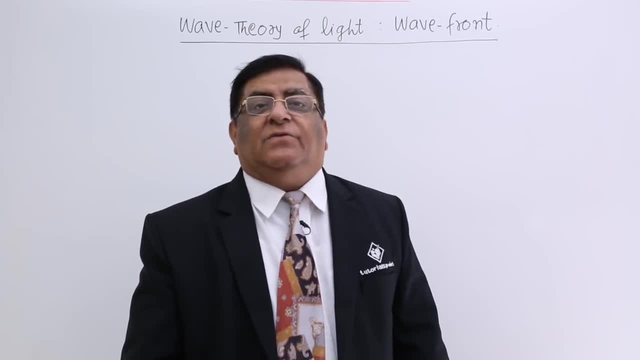 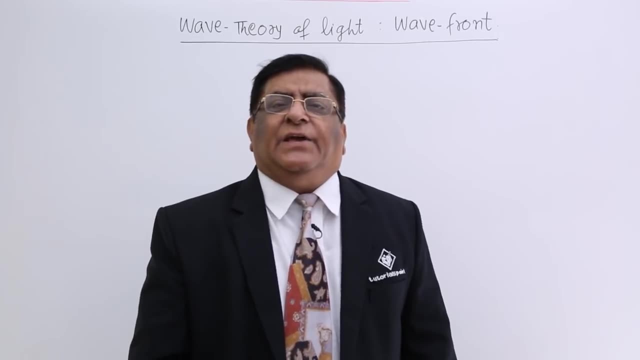 Ok, Ok, Ok. So, like all the waves in the world, there is an element which is the wave. So how can we explain that? So what is the wave like? what is the shape of the wave? Answer is very clear. 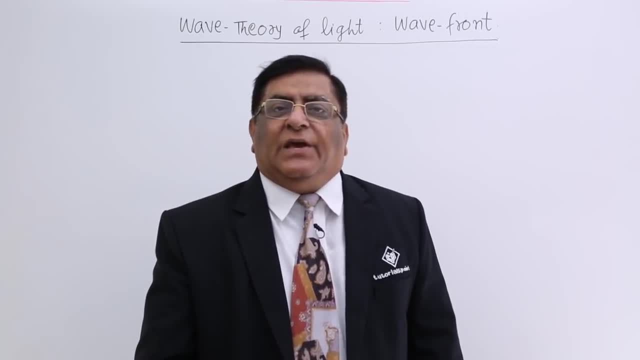 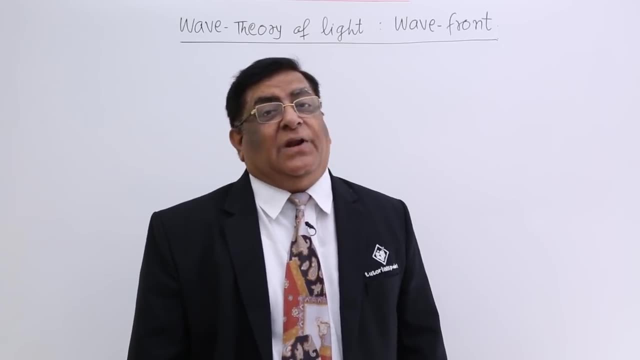 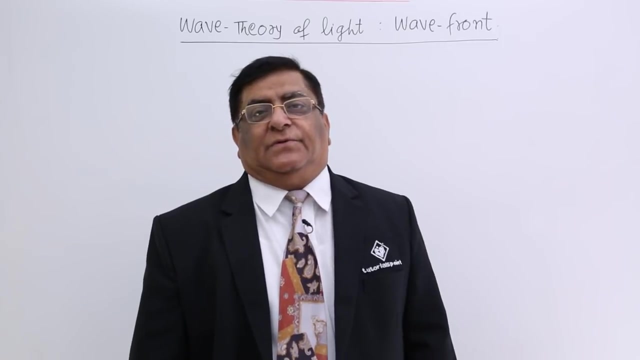 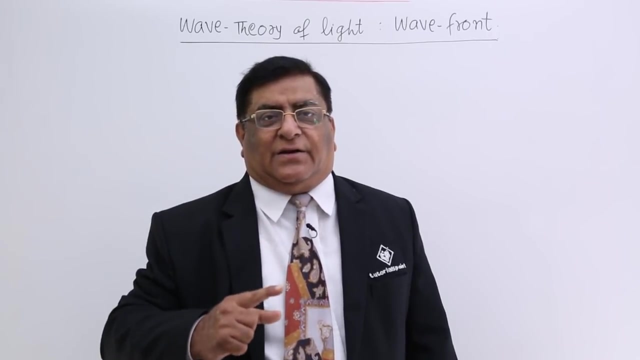 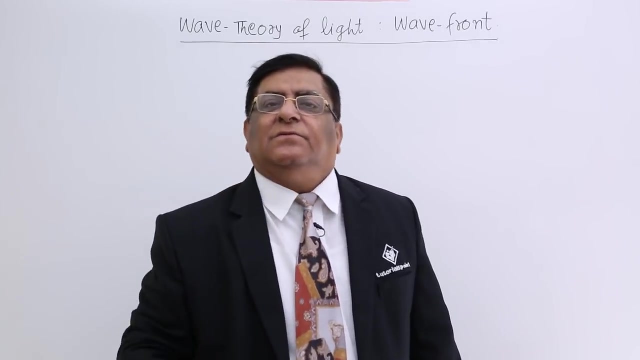 We have seen the waves of water, We have seen the waves on strings. So, similarly, there is a wave of light. Whatever material the light is made of, it travels in the form of waves. that means there are certain disturbances, and those disturbances are in that medium, in that material for which the 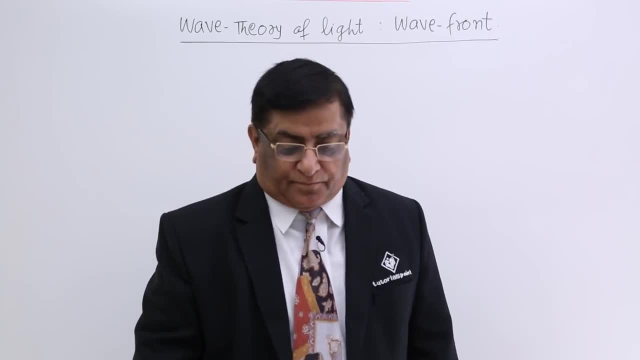 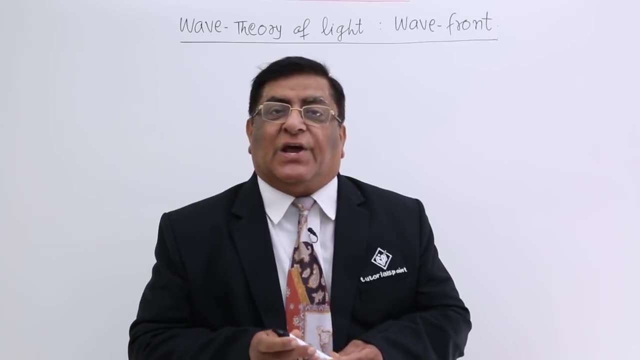 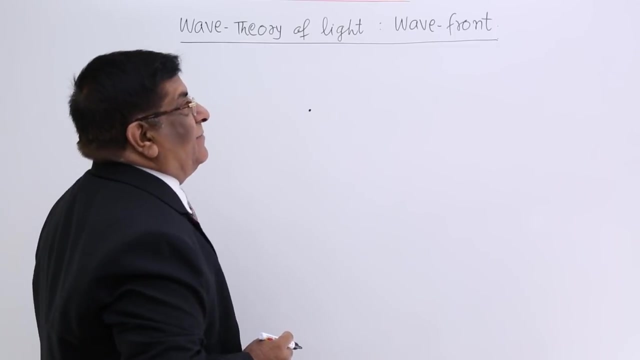 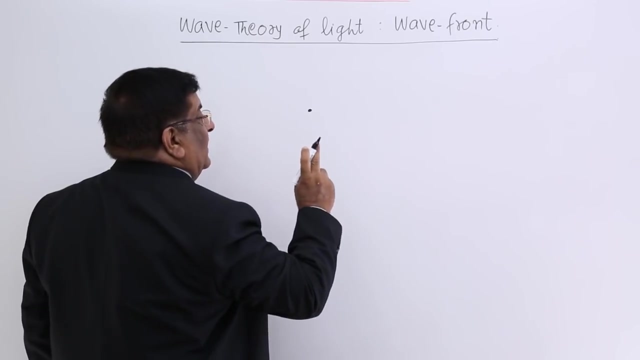 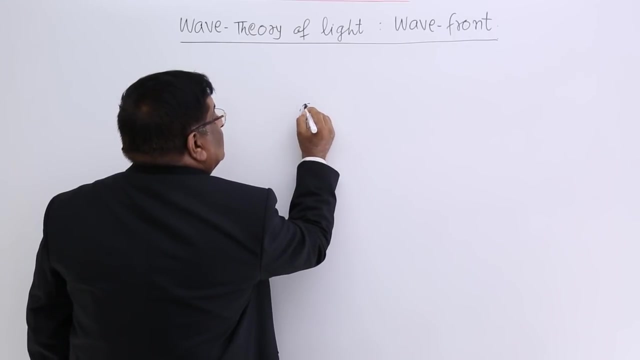 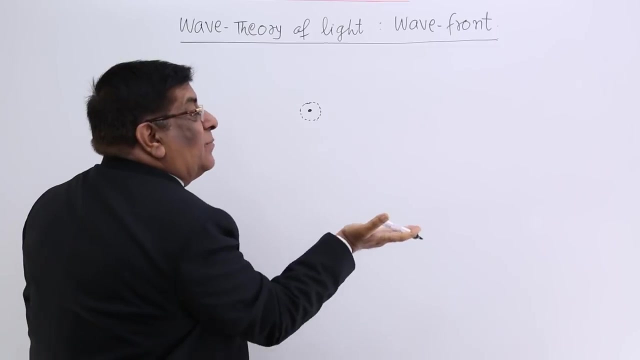 light is made of. Now he explained the waves in a manner we can understand it very well. There is a source of light which is created disturbance in the medium. Because of this medium, we have seen the water waves. There are certain particles of water here this, which have risen up the level. 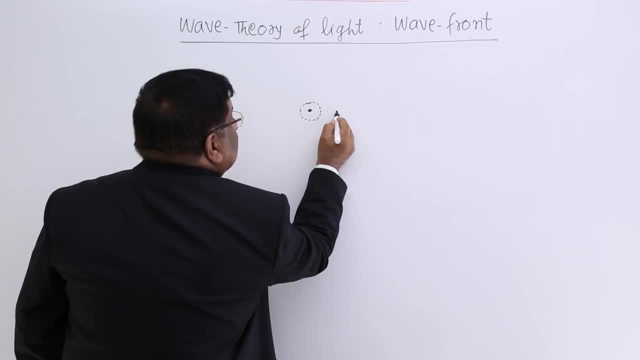 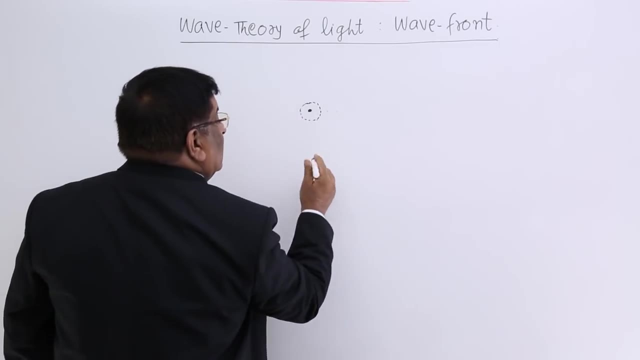 Then these particles have risen up the level, Then particles go down and these particles again up. So here are the particles. If I see them from one side, the section side, I find here are the particles which are down, here are the particles which are up, here are the particles which are down. here are: 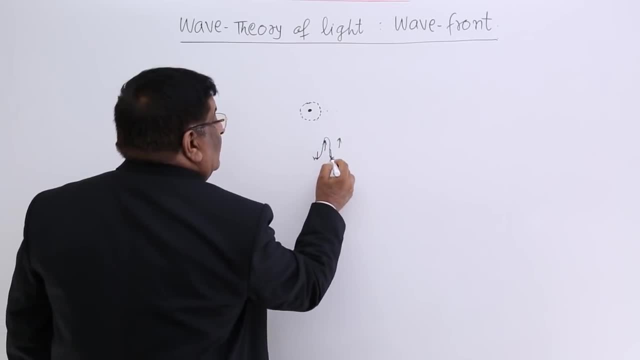 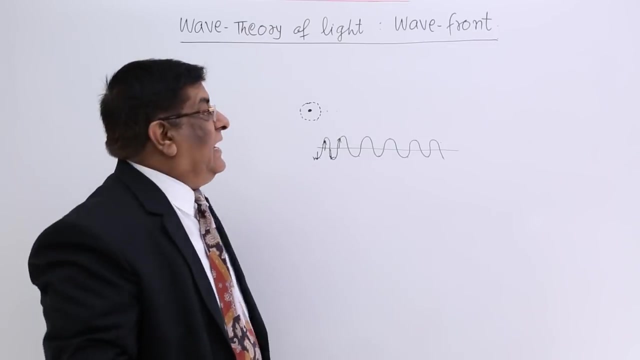 the particles which are up. So if I join them, I see this. So there are 3,000 particles. There are some places where the particles are up, there are some places where particles are down. This is general construction of wave and when this particle oscillate, it oscillates the. 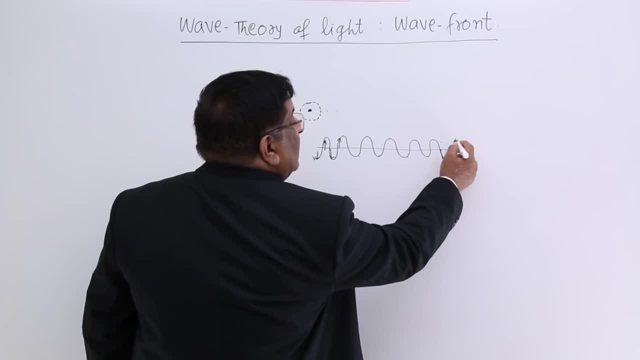 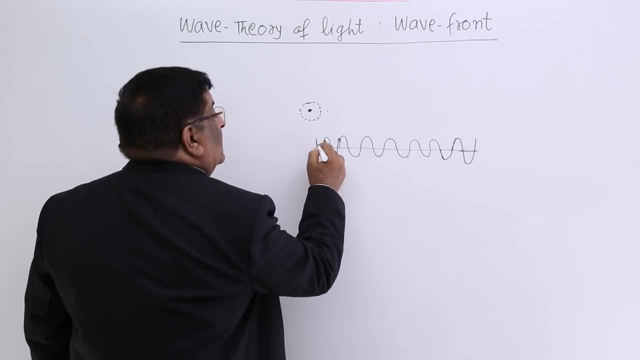 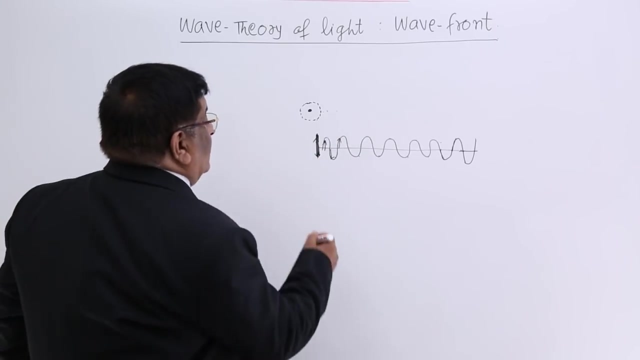 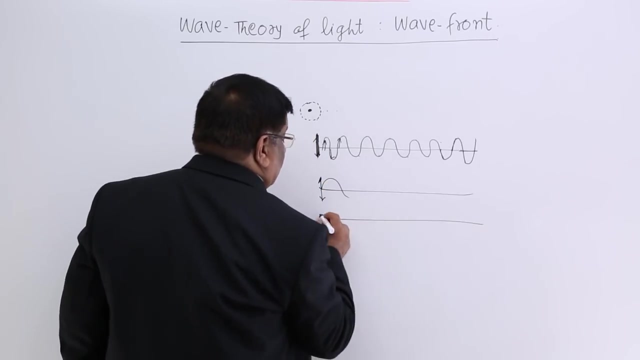 neighboring one. when this oscillate, it oscillates the neighboring one. when this oscillate, this oscillates the neighboring one, and this source, this keeps on vibrating here like this. So there are disturbances which was created at this place. This disturbance reach here after some time. it reach here after some time. it reach here. 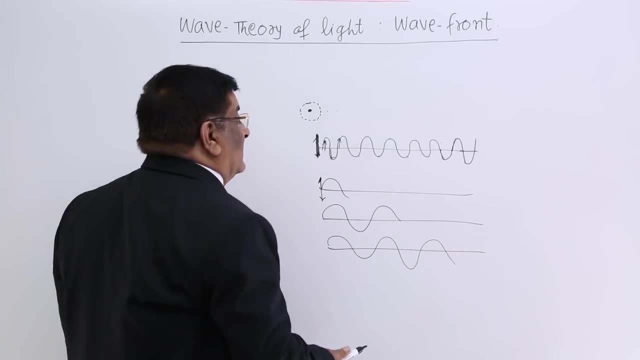 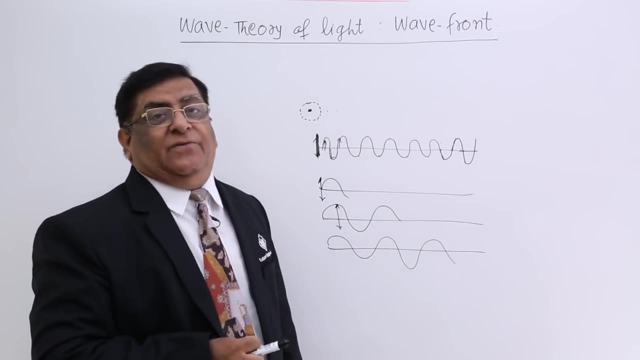 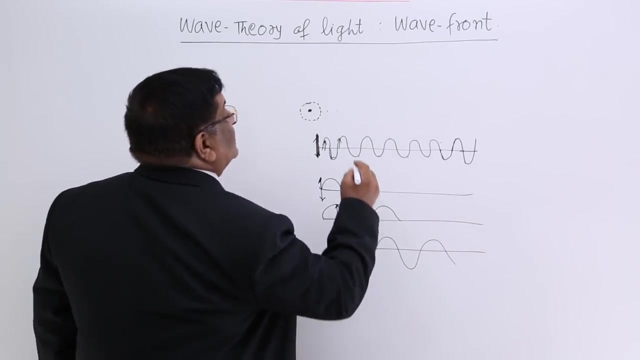 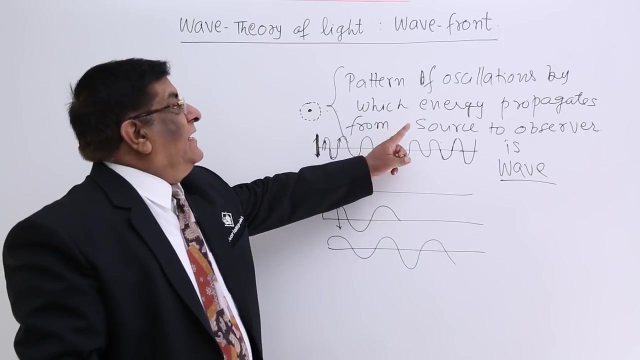 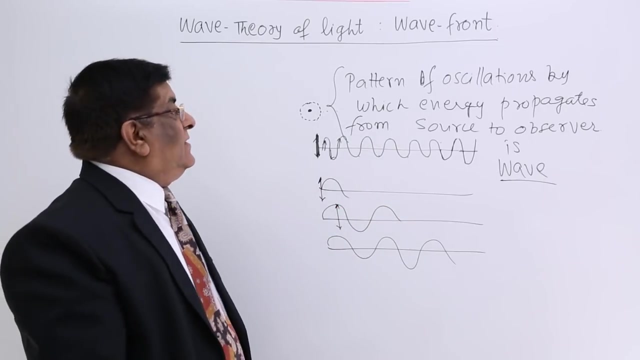 So the disturbance goes on increasing. and disturbance is what Disturbance is: oscillation of the contents, whatever it is made of. So this pattern, This pattern by which energy moves, is wave. This is wave, you can note it down. Pattern of oscillations by which energy propagates from source to the observer, that is wave. 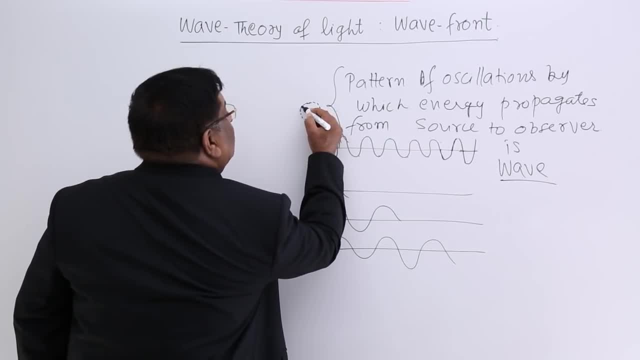 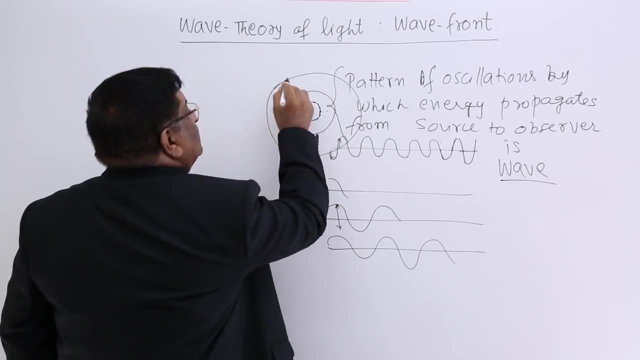 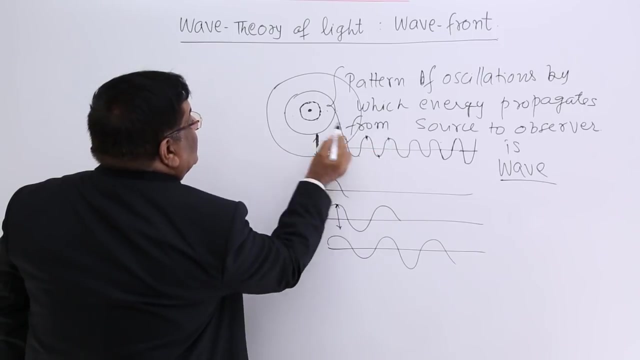 Now, in this pattern, we see something here: this, then this, then this. These are very important. If we see from the side, we see this portion is up up, this portion is down. this portion is again up. this portion is down. this is again up. 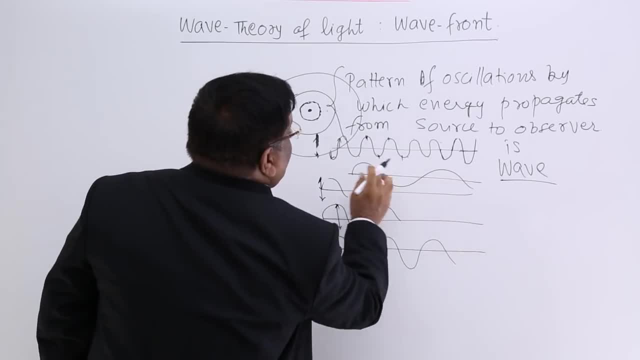 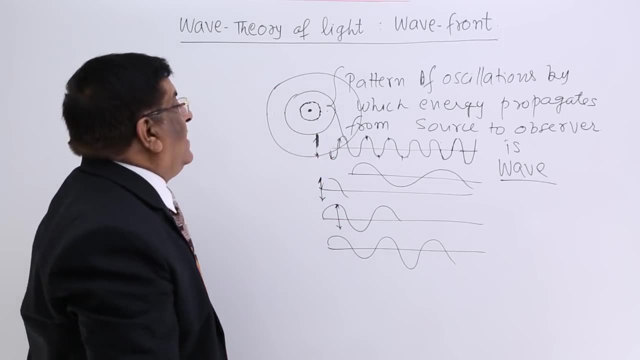 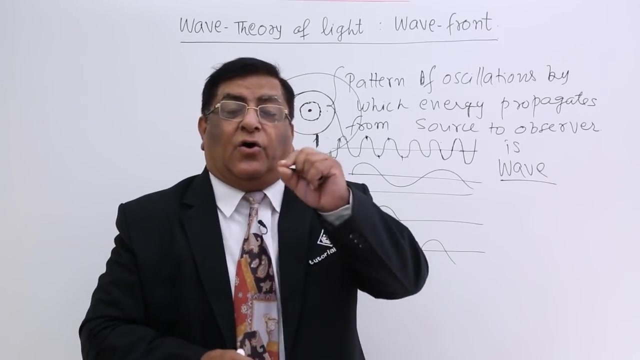 So we get a this way. This is from the side. we look like this. This is from the top of the water where we have thrown the stone. Now this is a one wall like structure, A wall like structure where all the points are up. 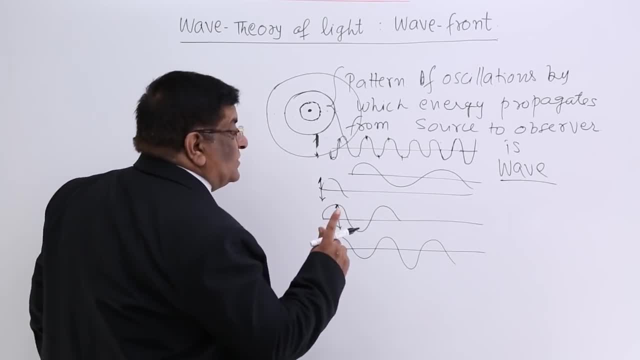 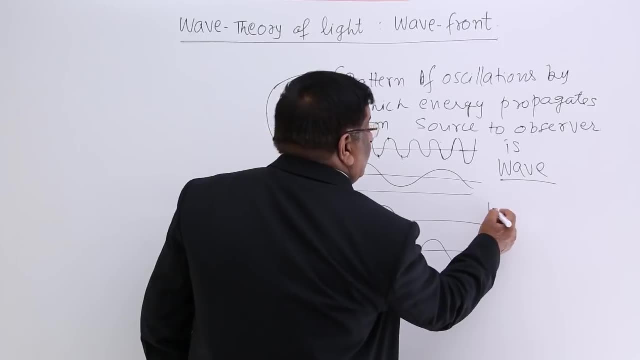 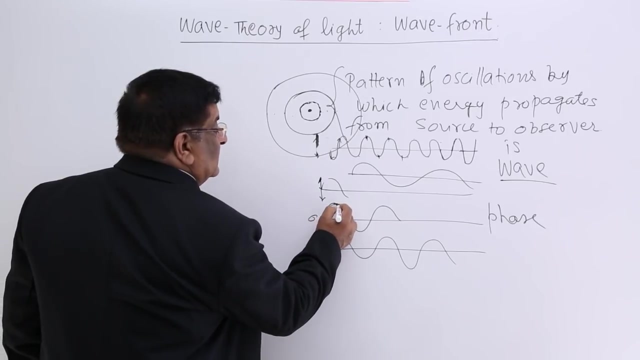 In the wave we have studied, the position of a point is termed, is given a term which we call phase. This is phase 0. This is pi by 2.. This is 1 pi, This is 3 by 2 pi and this is 2 pi. 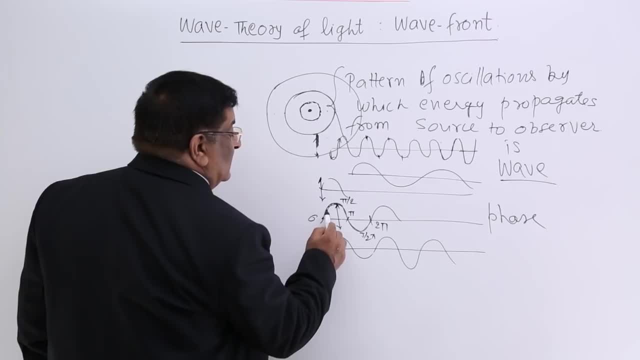 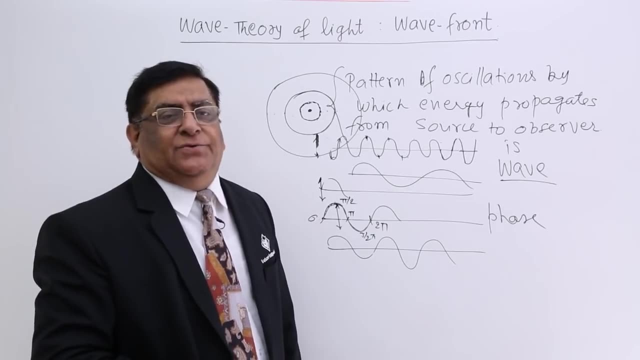 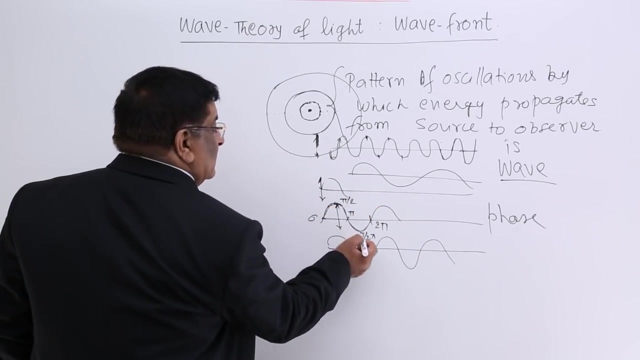 So this is how the phase of the change, at every point. If somebody ask me show me the phase pi by 2, I will show him this top portion which we also termed as. this is trough and this is crest. So this is trough. 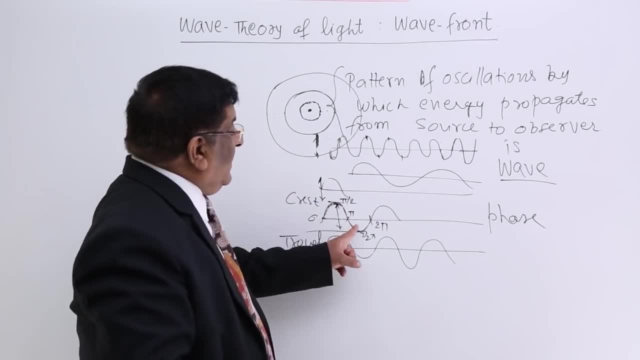 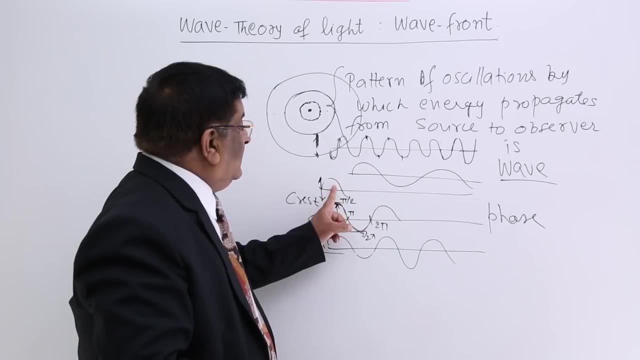 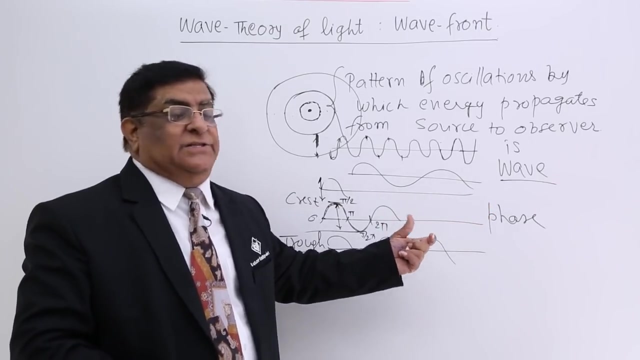 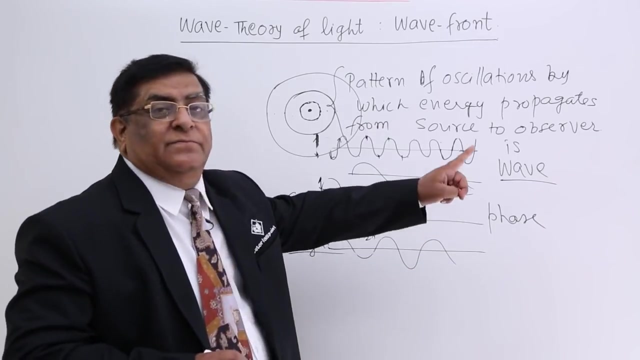 This is crest, This is trough. So the wave has a character like this: It moves forward in the shape of crest trough, crest trough, crest, trough keeps on making that, and all this is due to oscillations. So in this way, energy in the form of oscillations keeps on moving from one place to the other. 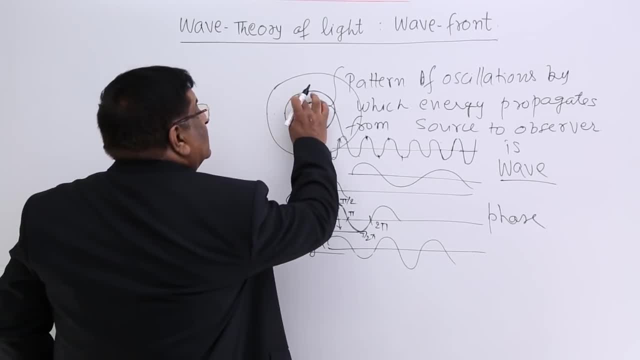 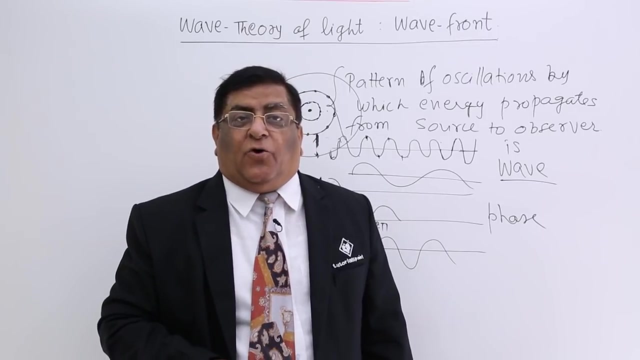 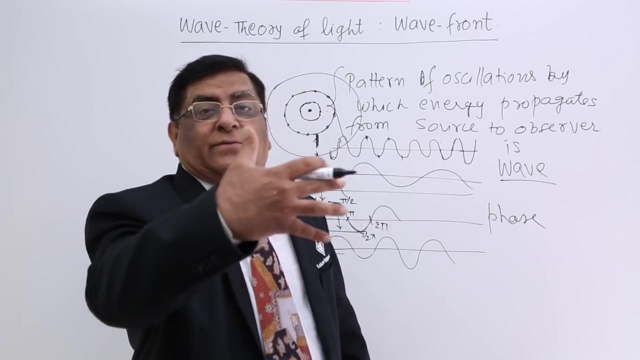 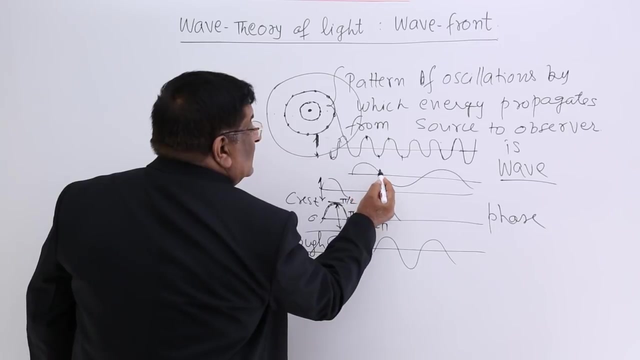 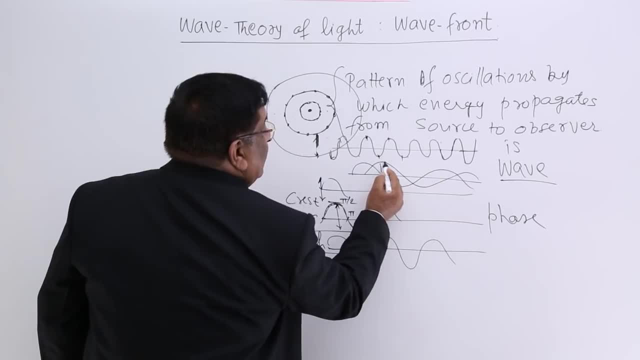 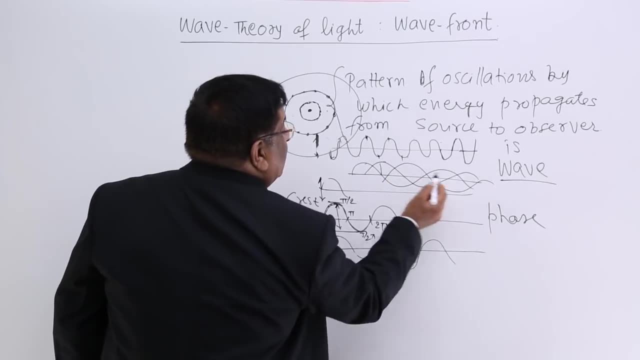 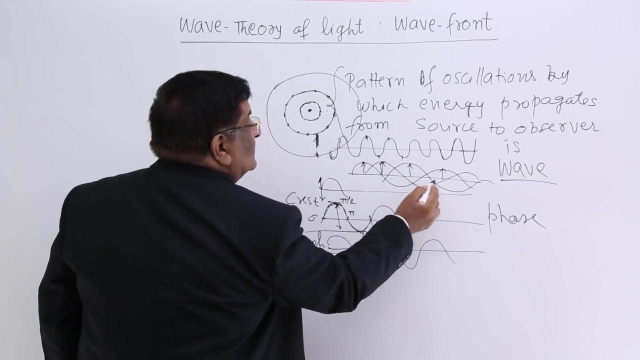 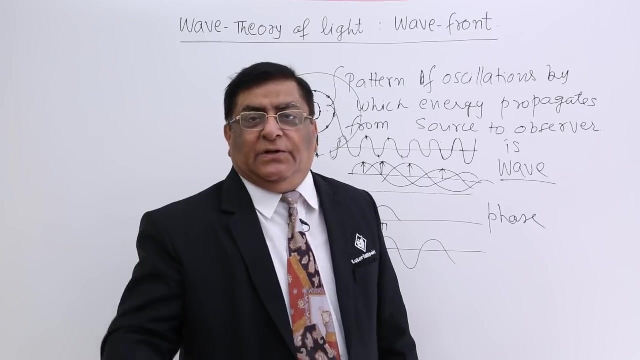 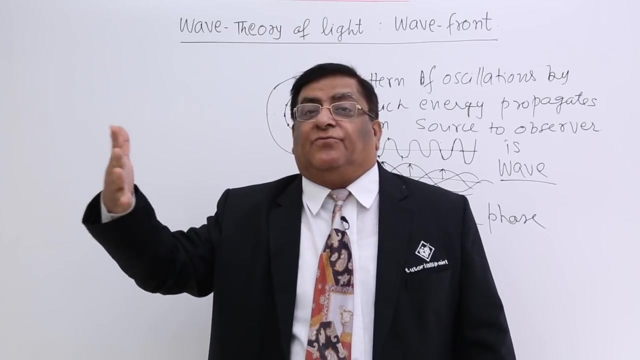 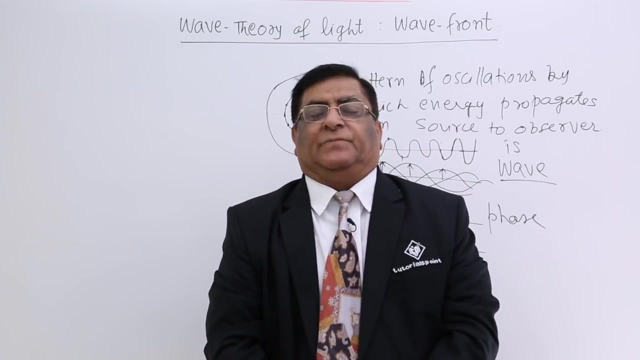 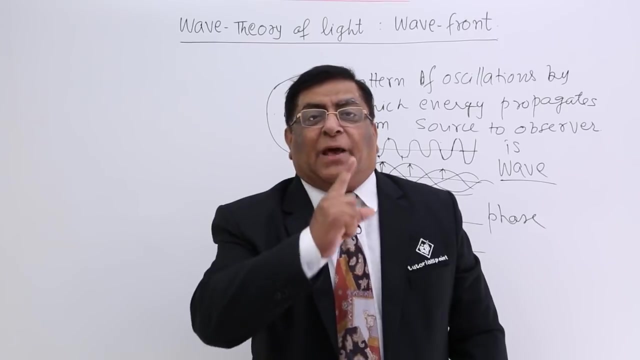 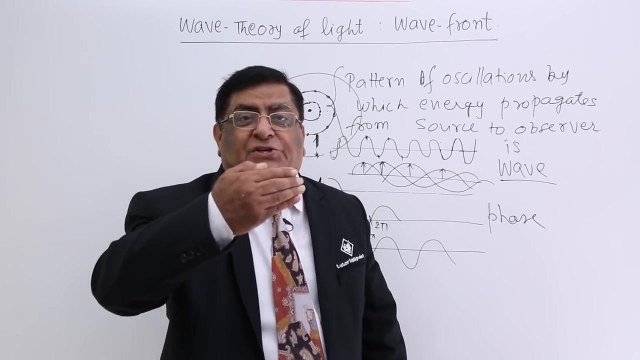 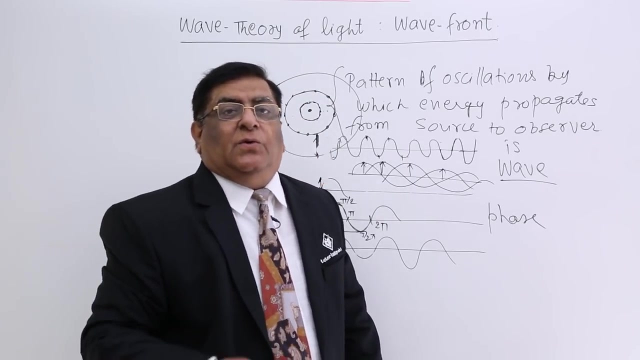 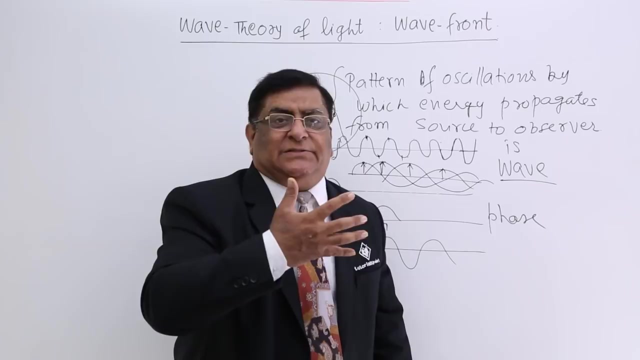 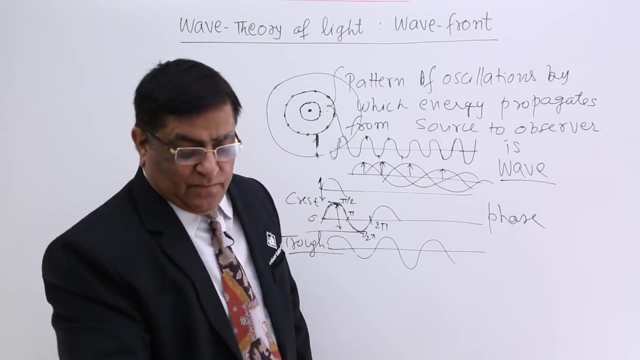 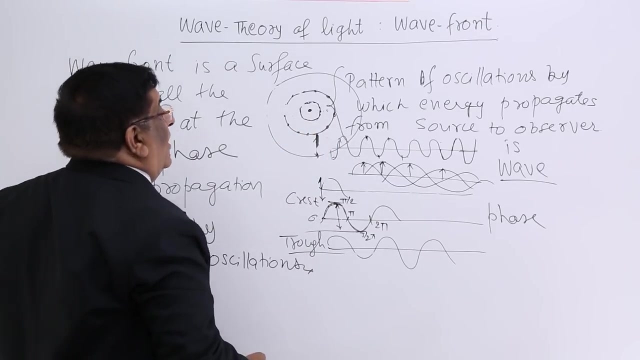 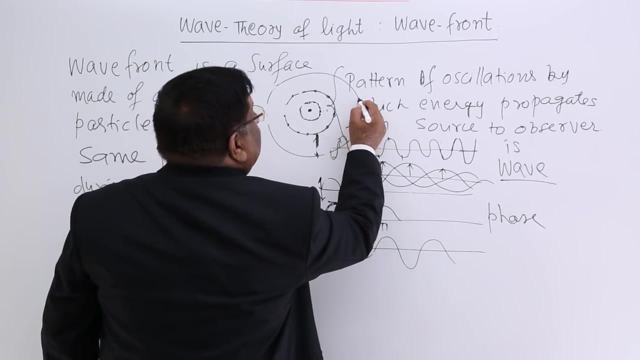 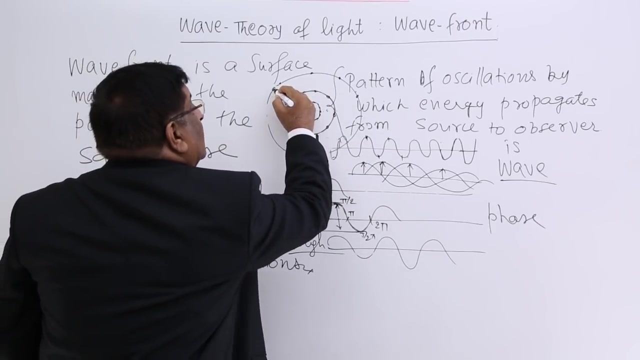 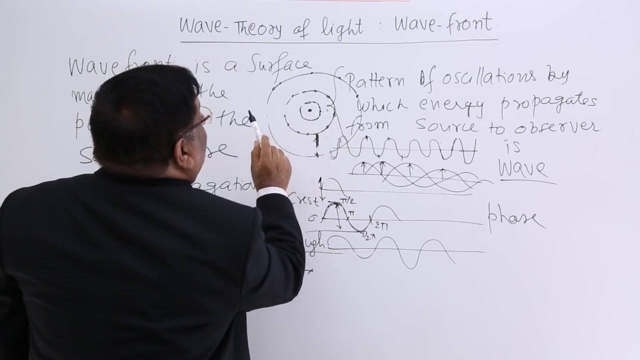 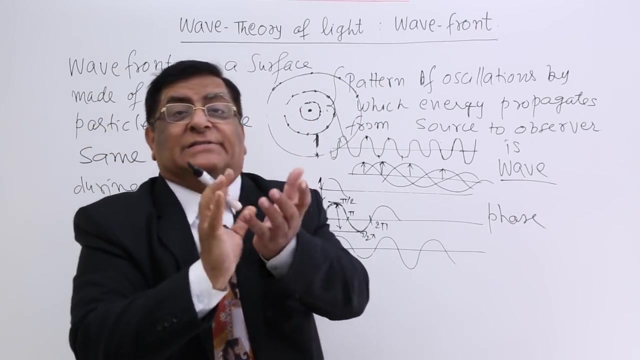 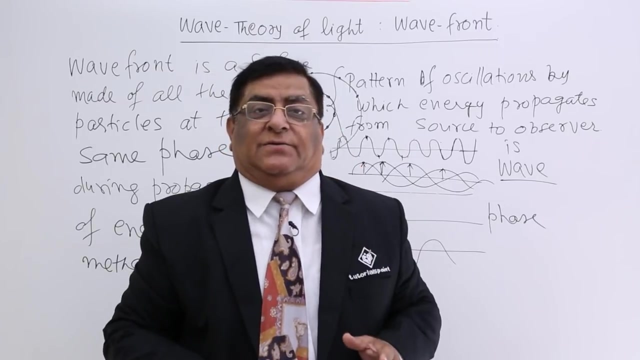 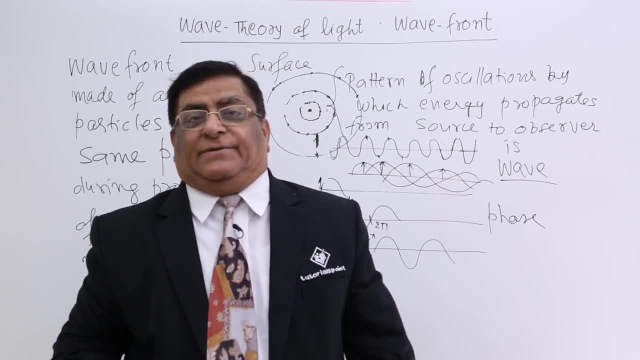 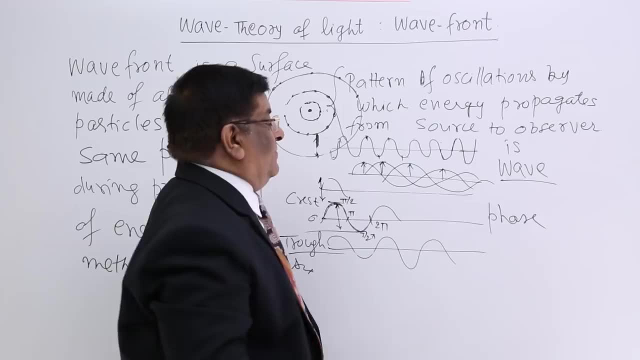 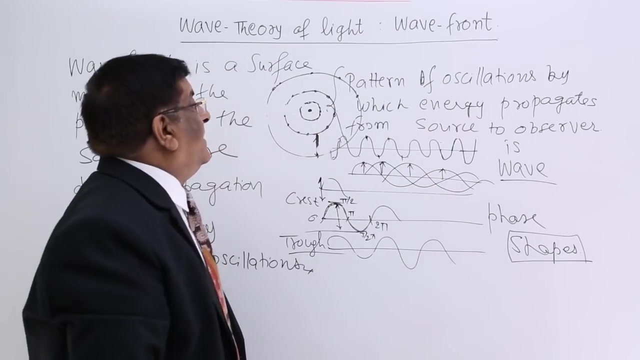 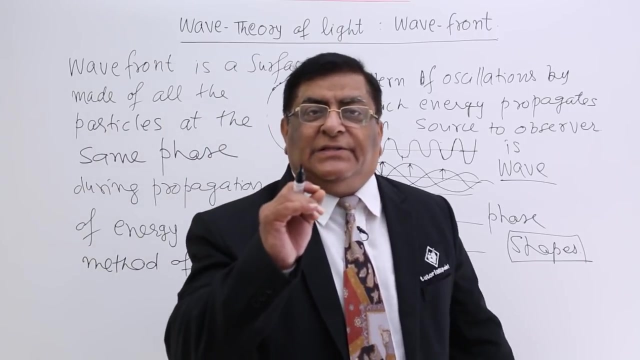 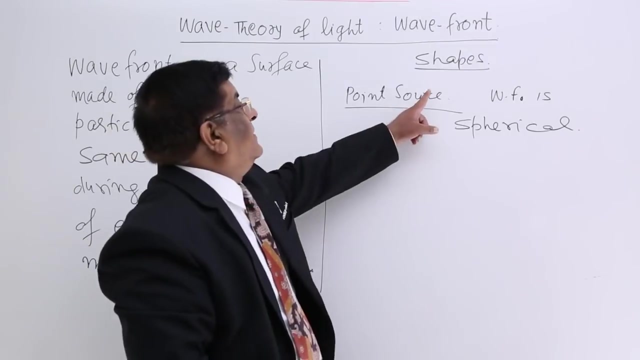 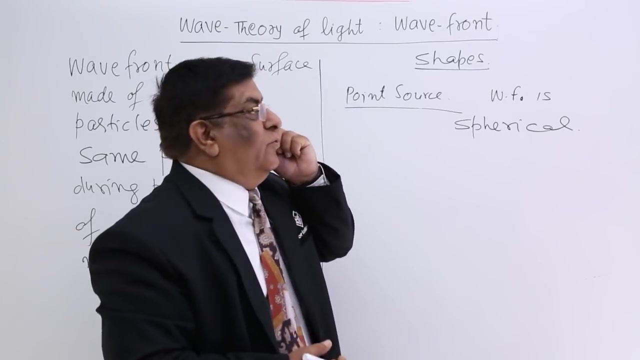 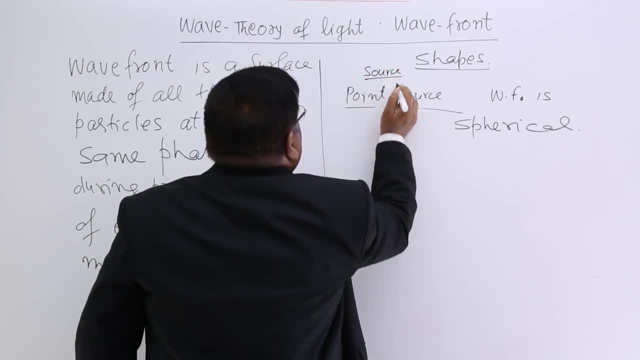 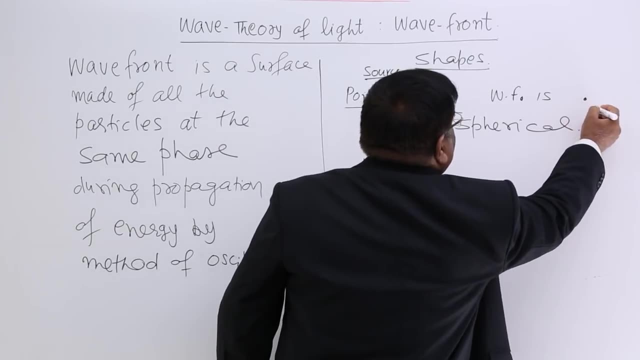 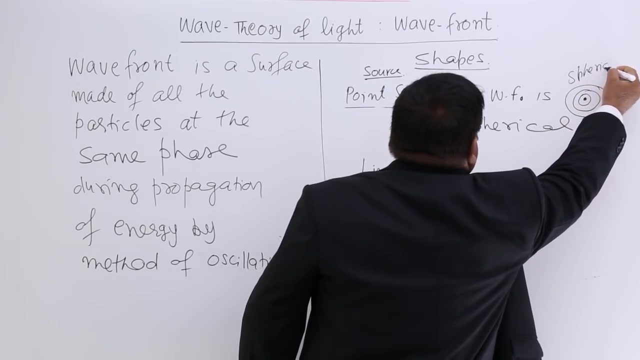 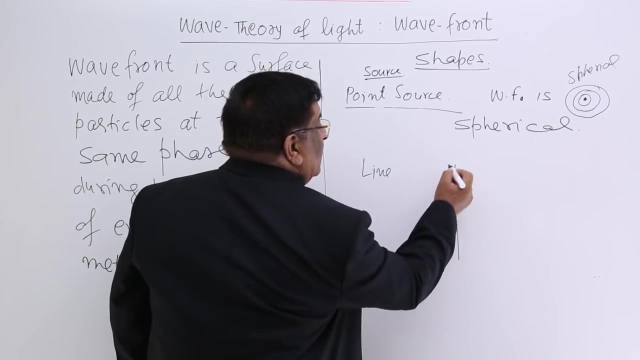 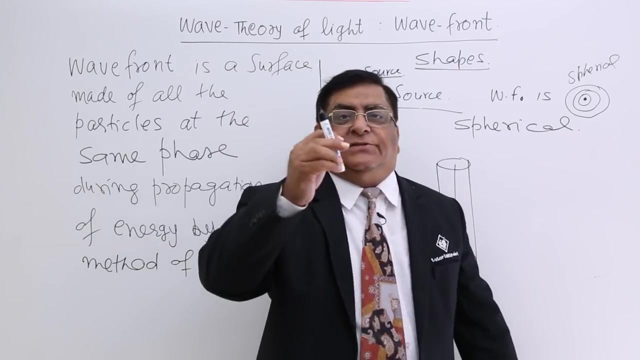 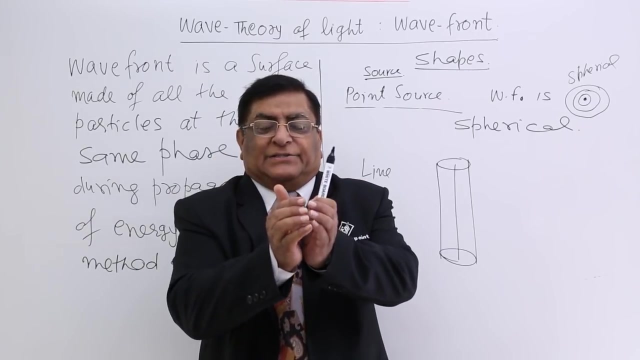 beschäftub slap outroớit. the source, and this spherical, this is what. spherical, that is the shape. ok, In case of line, this is the line and we get a, yes, cylindrical wave front. this is the source of light. there is one cylinder. after certain time there will be another cylinder, energy. 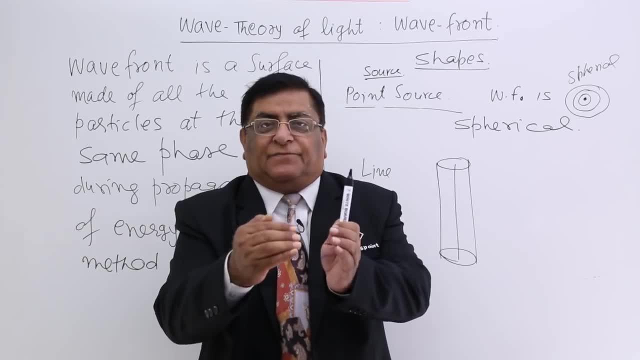 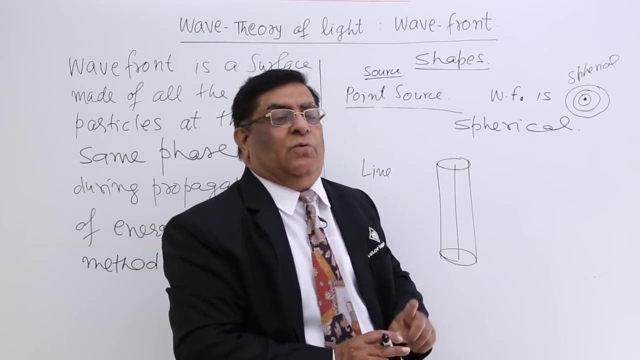 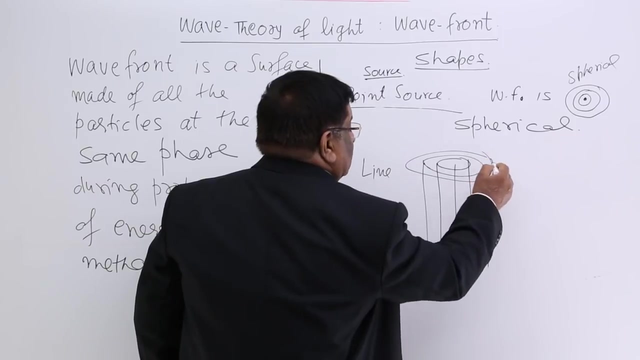 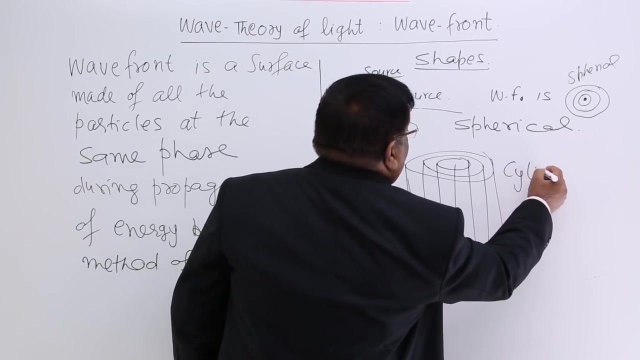 oscillations have reached this. after that, energy oscillation have reached this. after that, they have reached this. So what happens? cylinder after certain time, this cylinder after certain time, this cylinder. So these, this surface of the cylinder is cylindrical wave front, So cylindrical wave front. 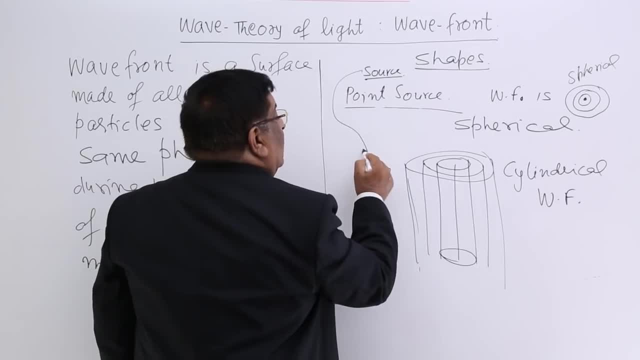 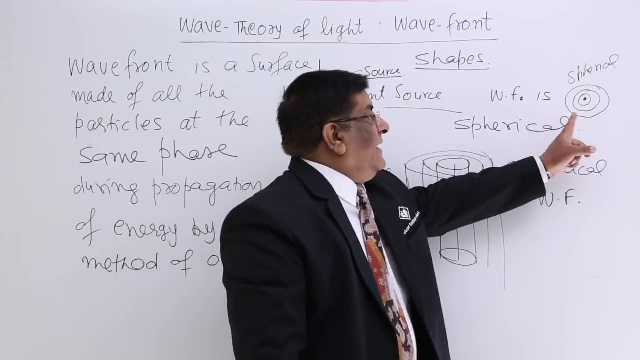 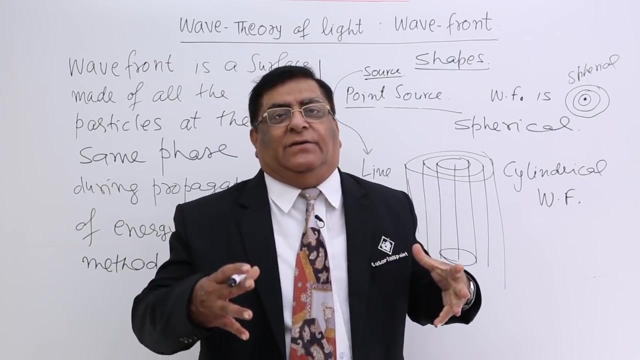 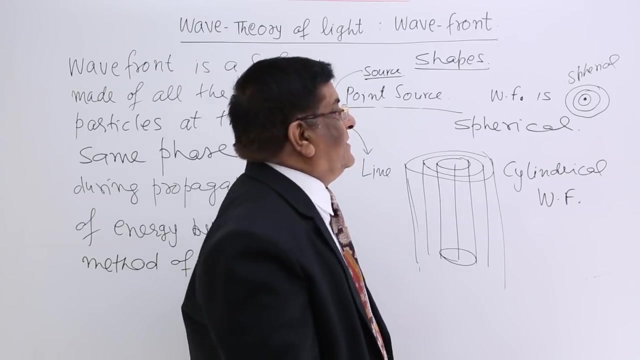 So cylindrical wave front is formed. when source is a line source, then whether it is a spherical, whether it is cylindrical wave front, the wave front is moving ahead. and what is the direction of wave front motion? and now comes a very important relation: in spherical wave front, the wave front is moving. 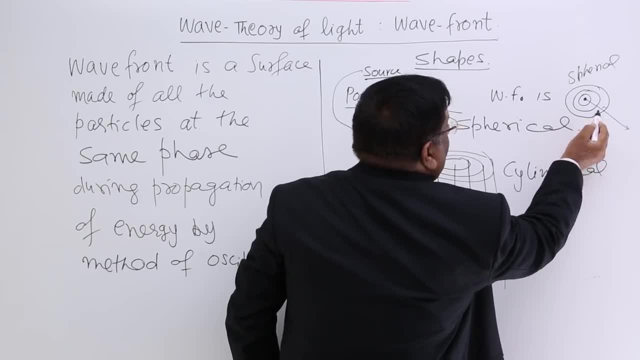 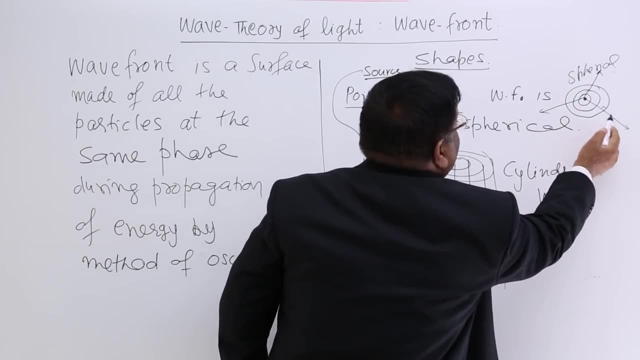 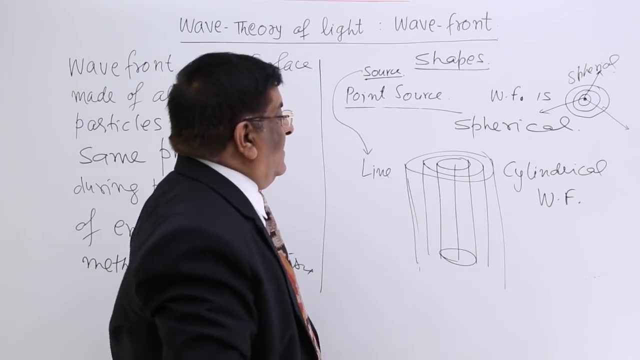 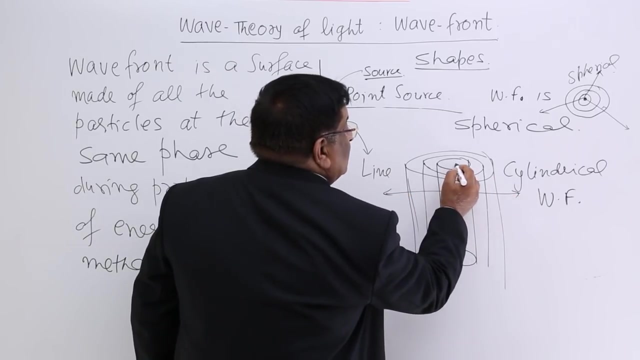 If it is moving straight, then movement is normal. Now may you imagine an object is moving in this direction, so am Kanalします ему or sabi har kurma masaber tul�� Chamber, out side of chamber, the direction direction, movement direction. If an object is moving in this direction, normally to this direction, if observer is here, then 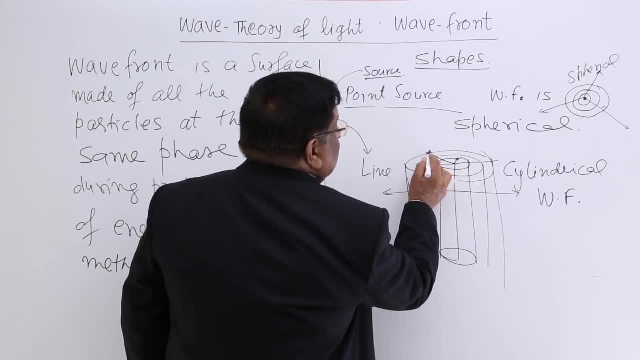 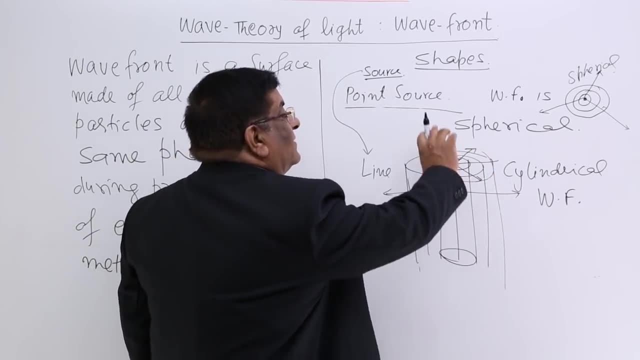 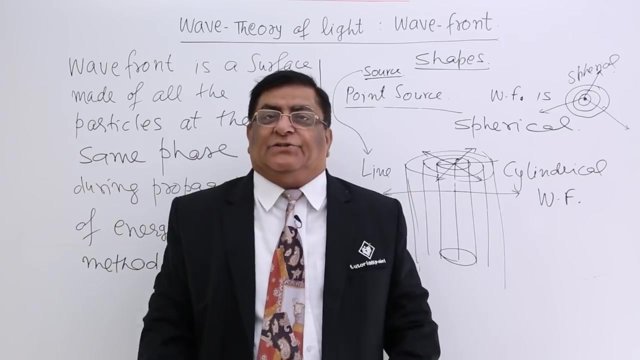 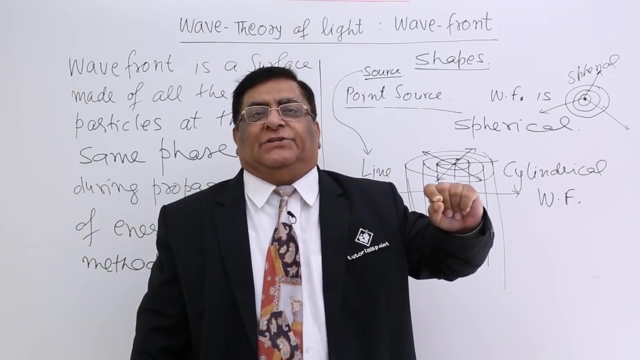 it is moving in this direction here, this direction. if we cut a section, we will find it is moving in this direction, but it is not going bottom or up, they are just moving like this, in all these directions. So now, the direction of propagation of energy is known as ray. 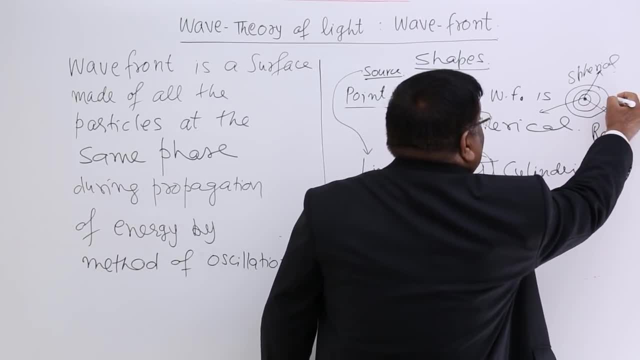 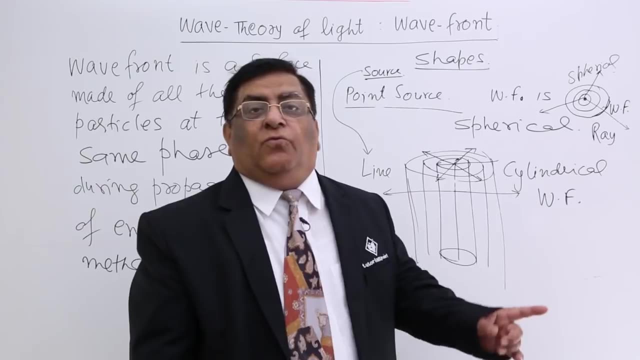 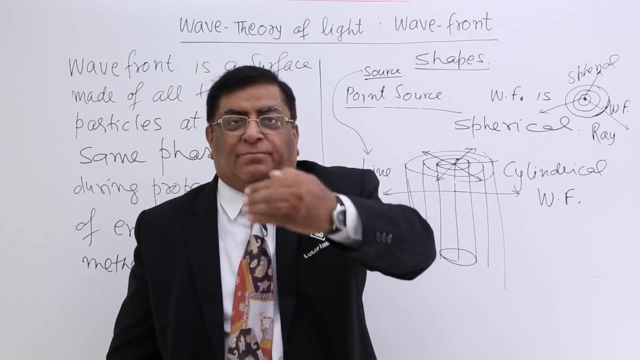 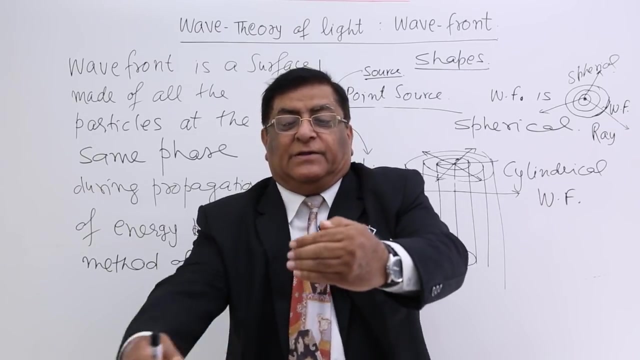 So this is ray and this one is wave front. So wave front and ray, they are perpendicular to each other. If this is a wave front made by this bulb, this source, this made a wave front, then next wave front, then next wave front, then next wave front. 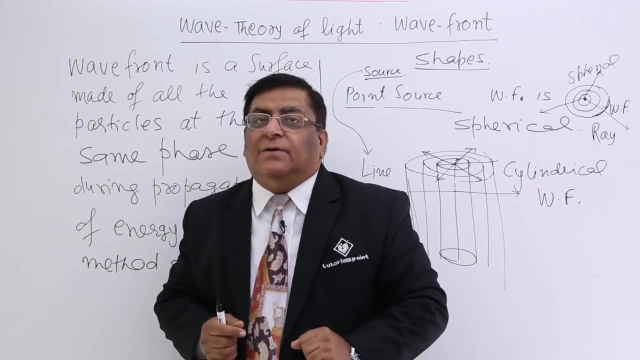 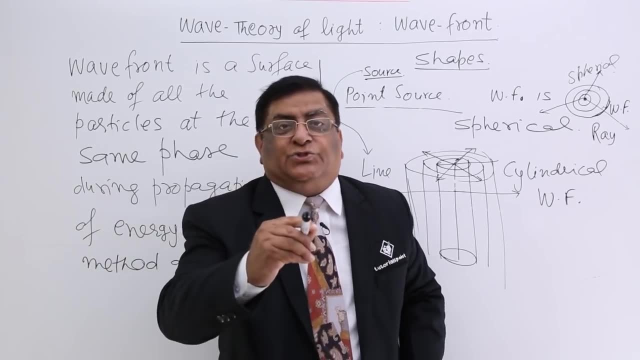 What is happening? The wave front is moving. The wave front is going to you like this: In which direction it is going? In this direction, See, in this direction it is going. So this direction of motion is ray and this is front. 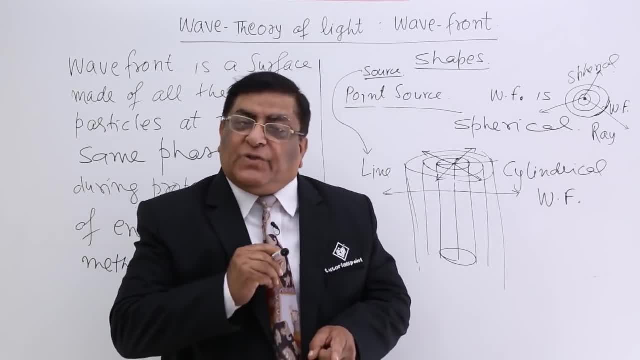 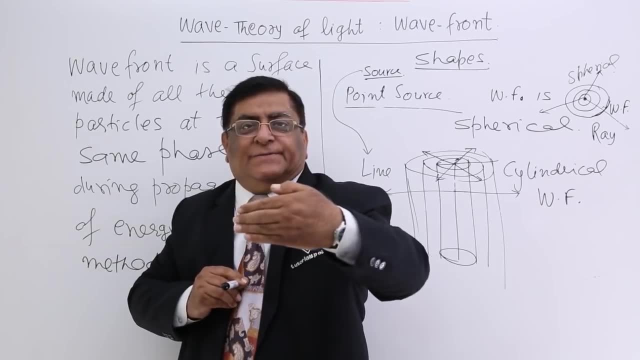 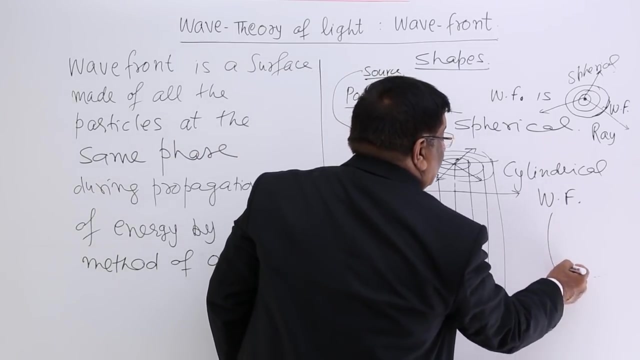 So this covers both our knowledge. The direction is ray and this is front. The front moves like this. So front and ray, they are always perpendicular to each other. If this is the front, then this is the ray and this is wave front. So ray and this and this is wave front. 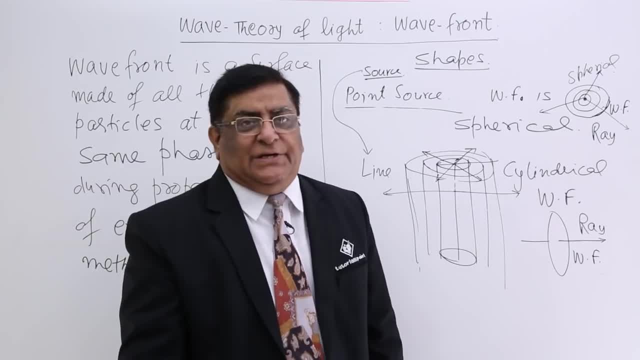 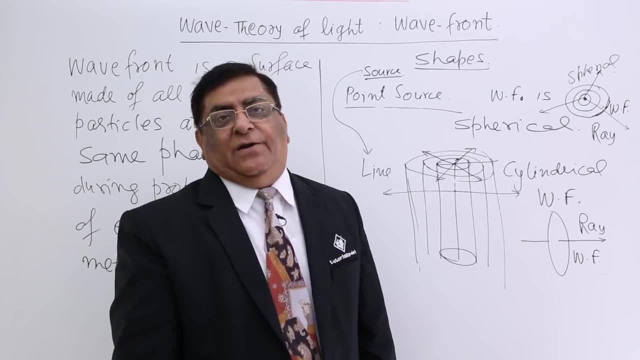 So wave front and ray are perpendicular to each other. so if we know the path of ray we can always draw the shape of wave front making perpendicular surface to the ray. If we know the direction of wave front, then here we will know that. if you know the direction, 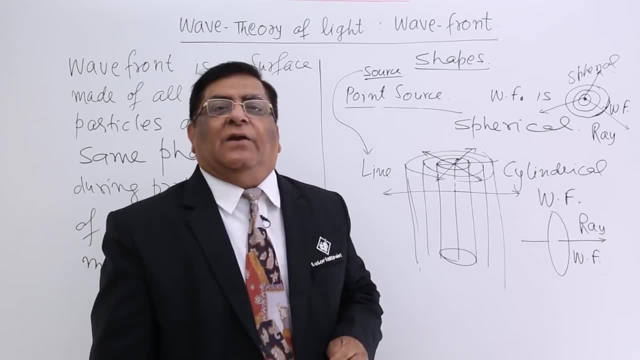 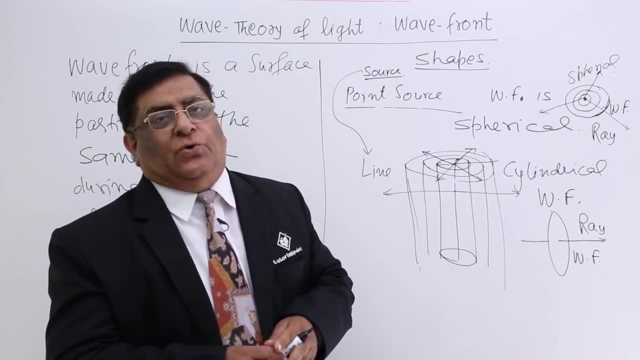 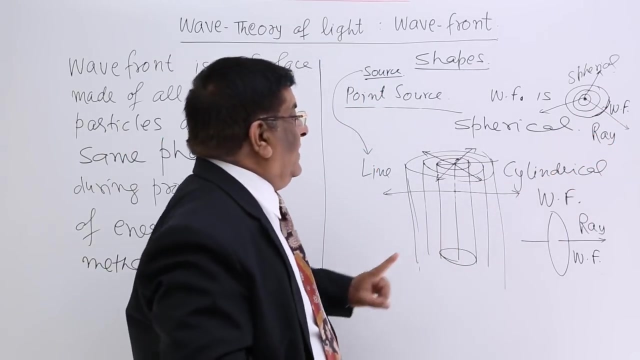 of ray. We couldnot draw the consistency. We can draw the wave front. we can always draw the direction of ray, making a line perpendicular to the wave front. So a spherical wave front has radial rays going out. Here we have it this way: cylindrical wave front. 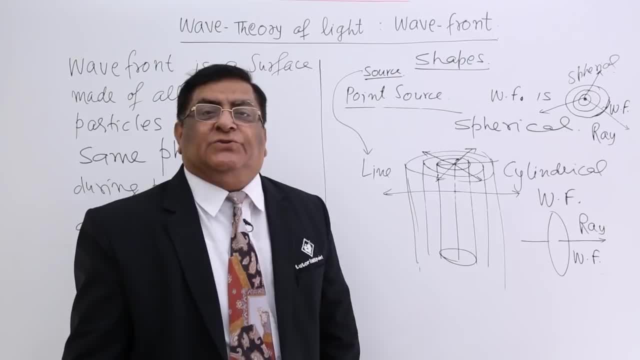 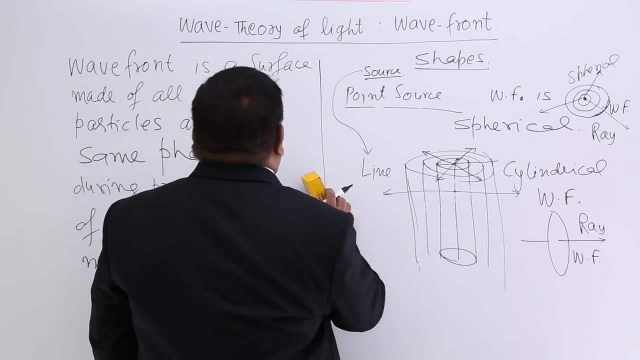 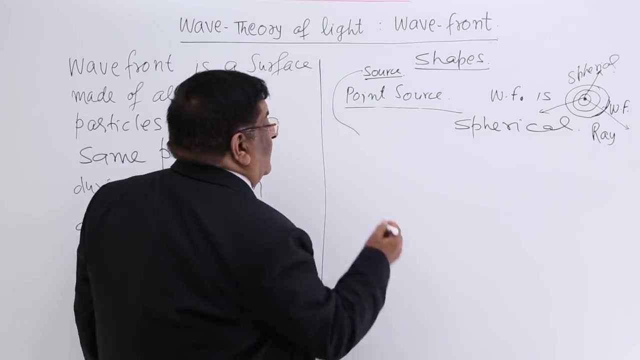 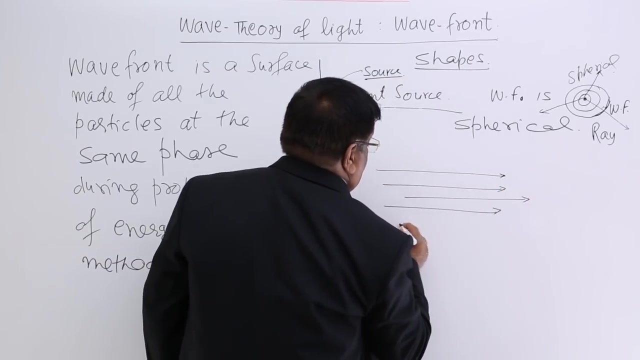 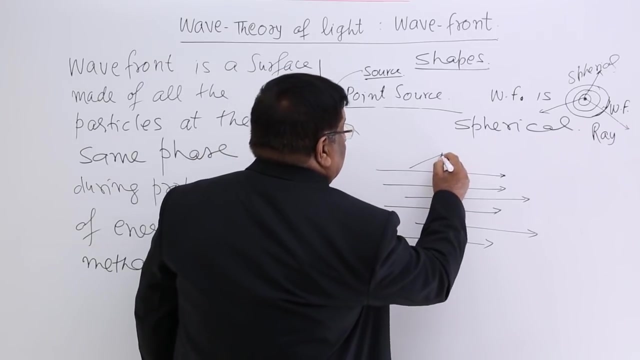 Similarly, if our source is far away, how the rays are coming. Answer: it is so far away that the rays coming become almost parallel. So if the rays are parallel this way, then where is the wave front? The answer is: this is the wave front. 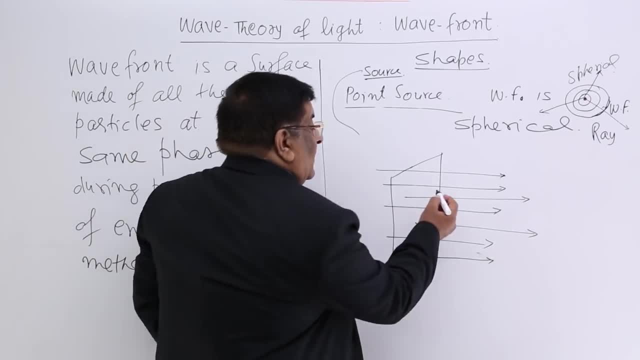 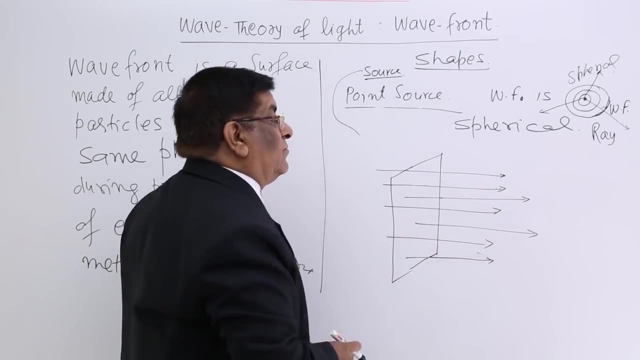 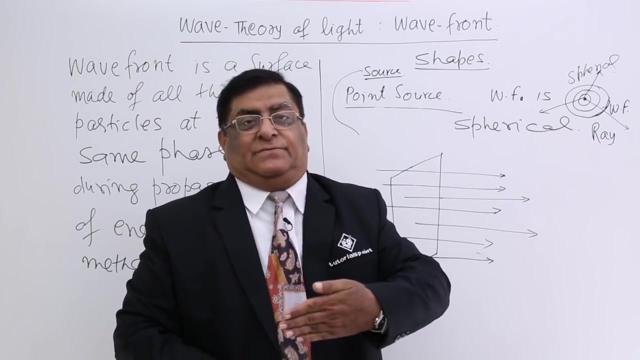 This wave front. here it is normal to the direction, Here it is normal to the direction, Everywhere it is normal to the direction. How it is possible? It is possible only if this wave front is a plane surface. So if this is the wave front, this is approaching you like this. 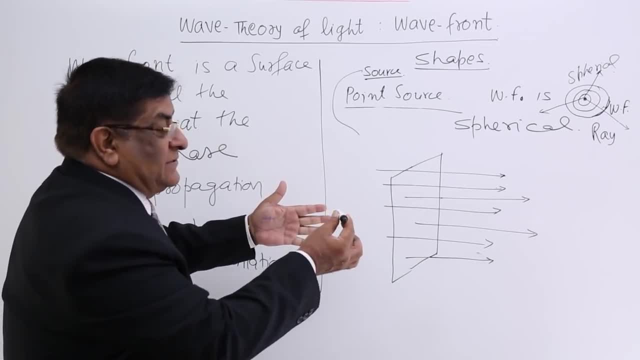 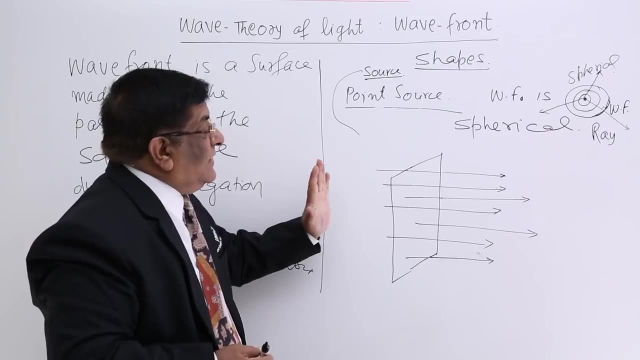 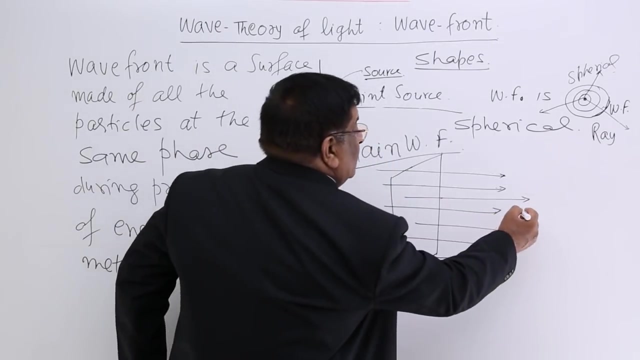 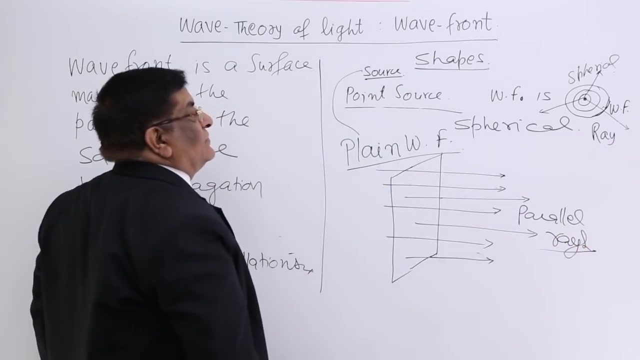 What is the direction of approach of this point This, This point, This, This point, This? So in this way, the rays are parallel, The wave front is plane wave front And these are parallel rays. So when the rays are parallel, the wave front is plane wave front. 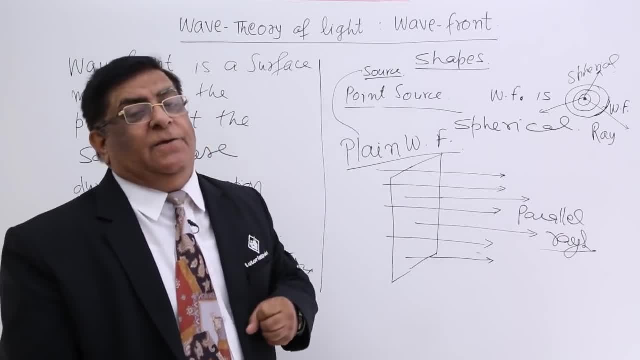 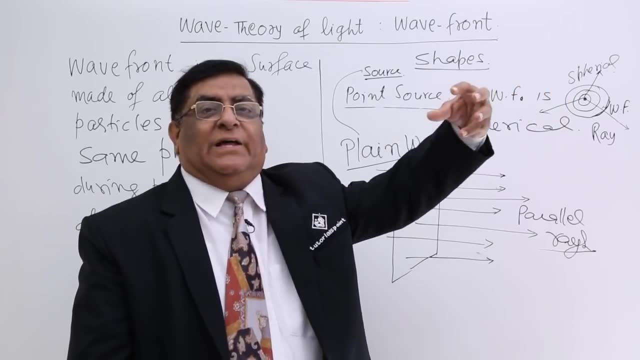 And this is the wave front we are going to use, mostly because sun is our main source of light. It is far away And from there, when the rays are coming, they are, so they are supposed to be parallel. If they are parallel, 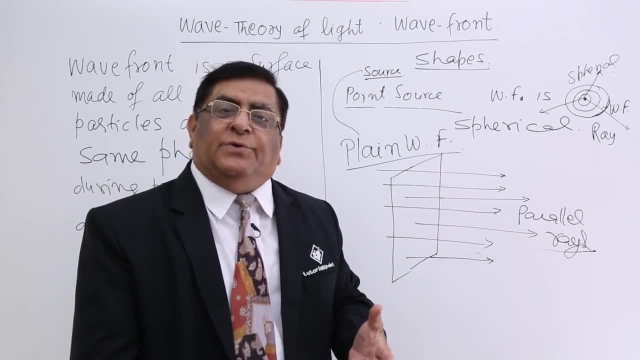 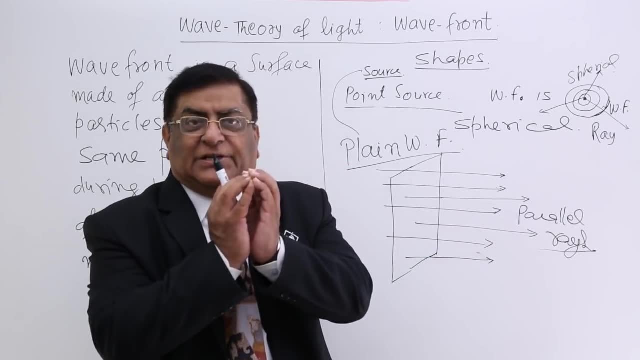 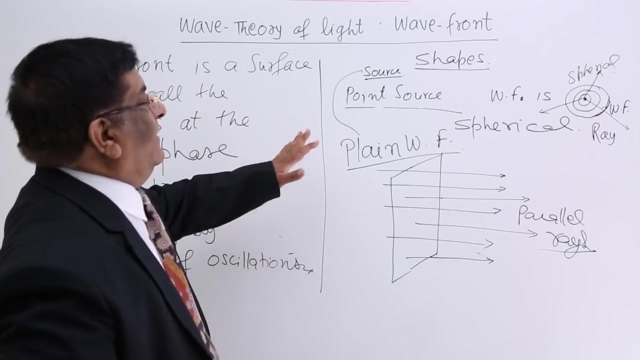 then the wave front coming from the sun is supposed to be a plane wave front. So whenever source is far away compared to the area in consideration, then we say the wave front has become plane. Okay, So that is plane wave front. spherical wave front. cylindrical wave front. 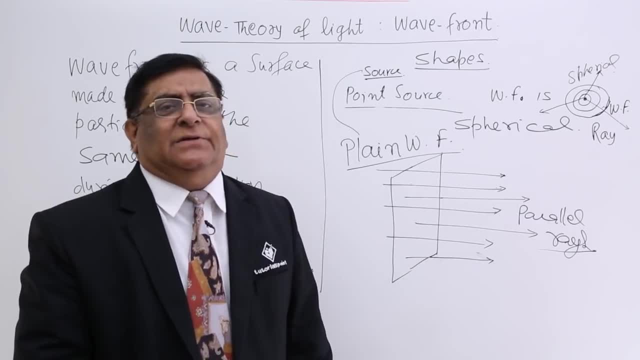 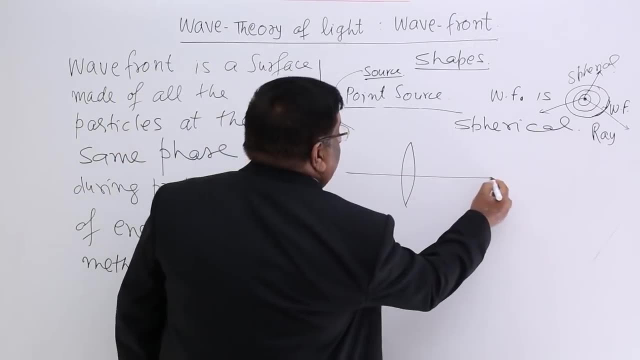 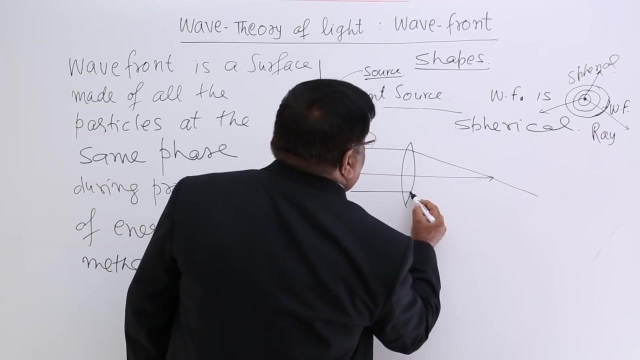 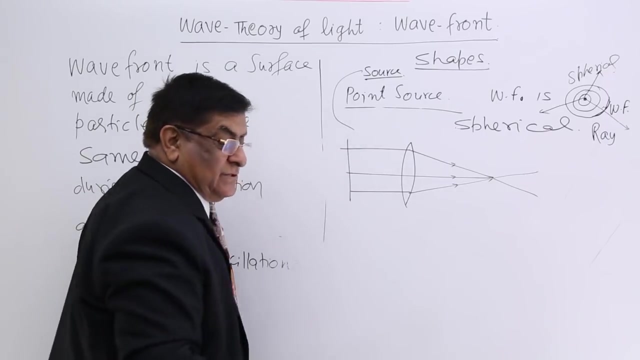 And then we have many different type of wave fronts And all we can find out- Concave wave front, convex wave fronts- How those can be a lens. This is a converging lens. These are direction of the rays. These are plane wave fronts coming from here. 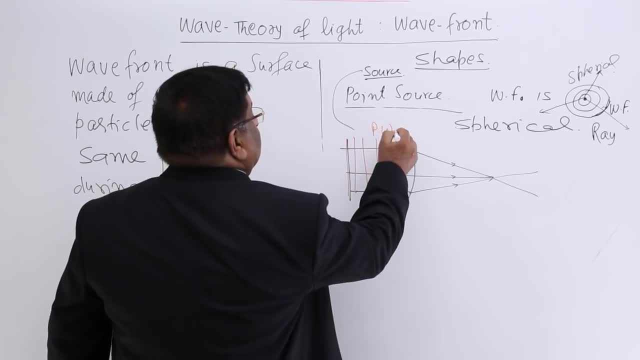 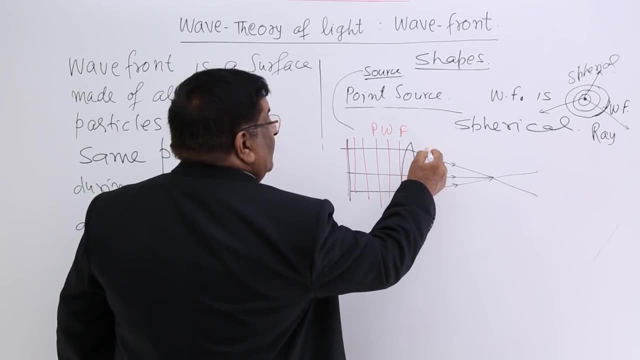 Plane, wave fronts Which are moving in this direction And once they reach here, after that, these wave fronts, normal to this, normal to this, normal to this, they become like this, They become like this way, They become like this. 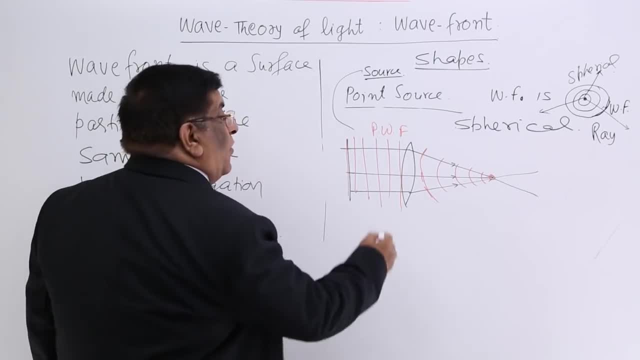 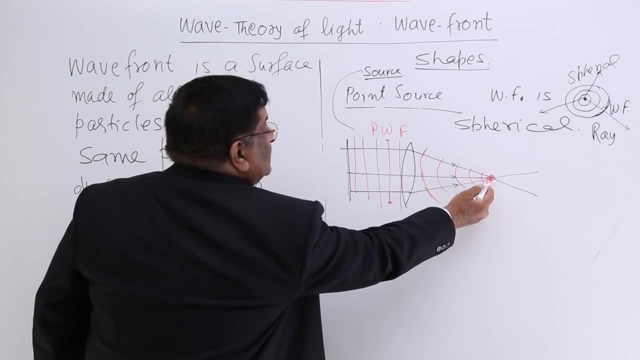 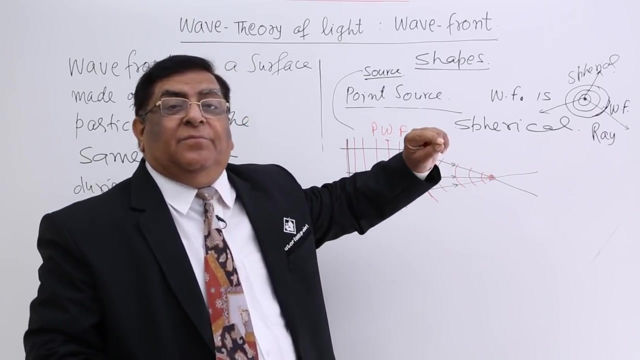 This, This, This. So all the energy filled in this long wave front has become in such small wave front. So the concentration of energy is very high And this appears to be a very bright spot, Because the whole wave front energy is now in a small wave front here. 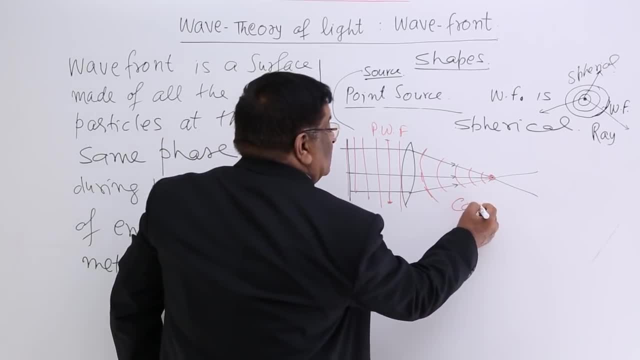 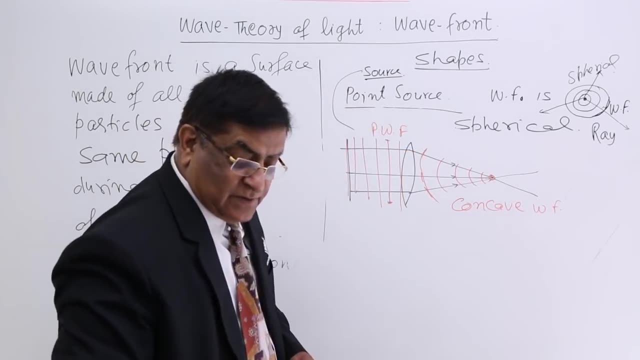 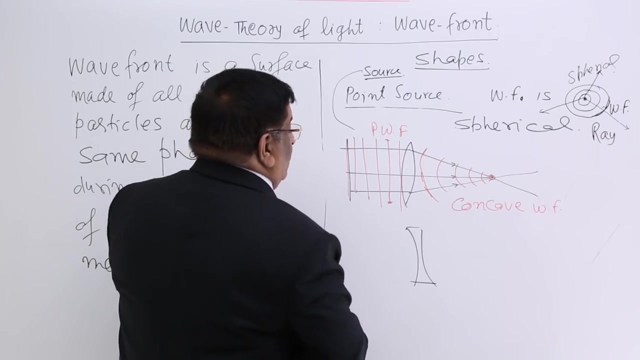 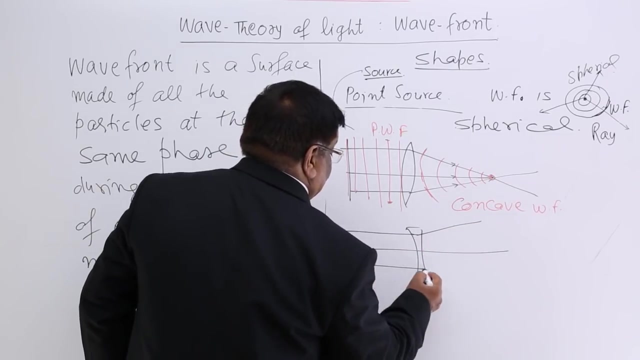 And this type of wave front is known as concave wave front. Who has made it a convex lens? Similarly, if we have a concave lens, what does it do with the wave fronts? We will first find out. what does it do with the rays? 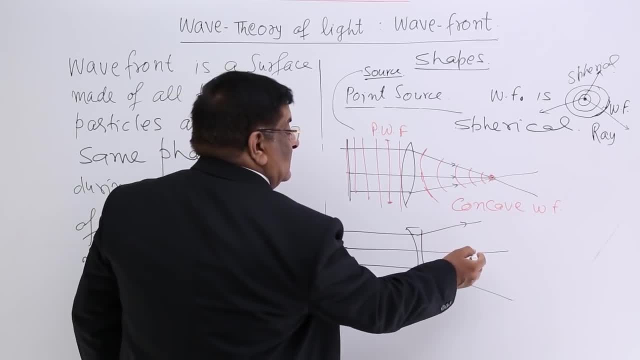 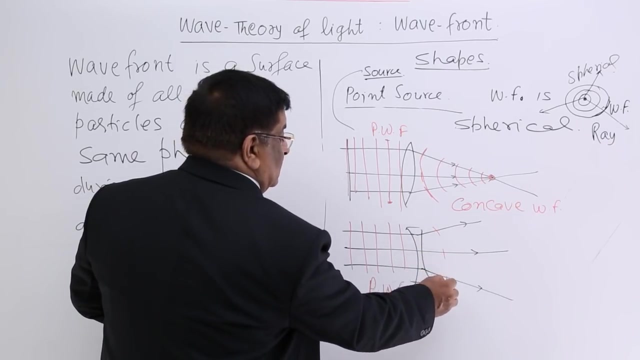 Diverging the rays. Now, if we make perpendicular, here is the wave front. This wave front is a plane wave front And after passing through this, this becomes this, this, this. This is a diverging wave front or a convex wave front. 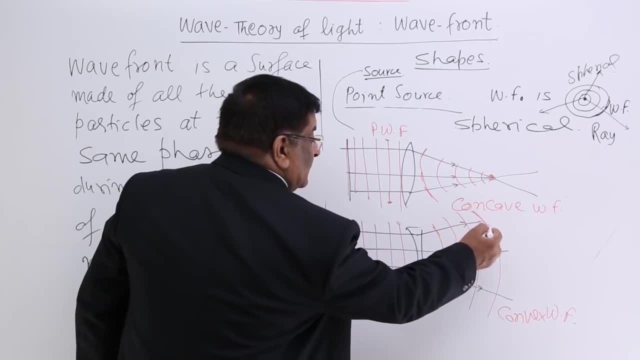 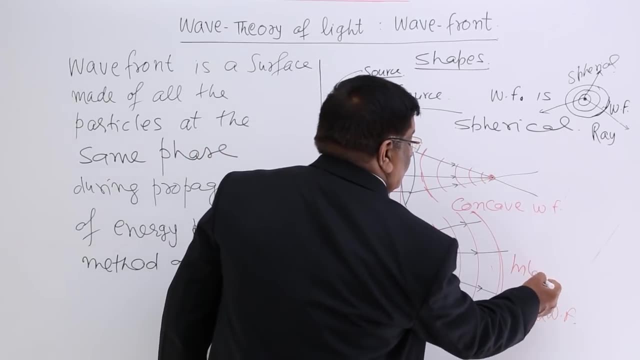 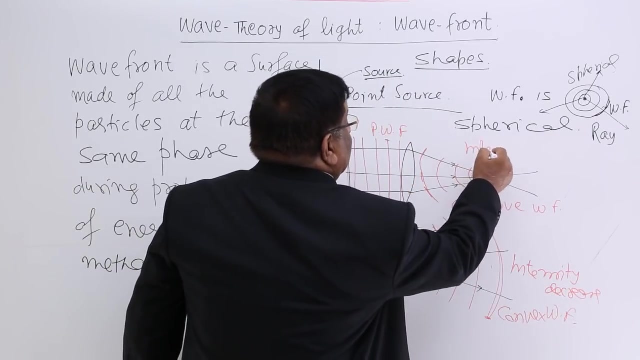 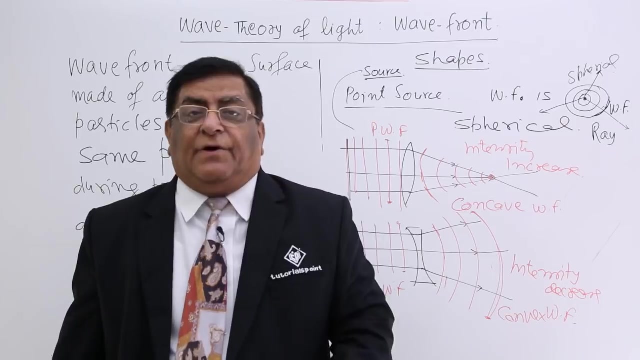 The energy which was carried within this is now distributed all over this, So the intensity of light become less. Intensity decrease Here intensity increase. So we have seen different type of wave fronts And how the wave fronts propagate in any source. 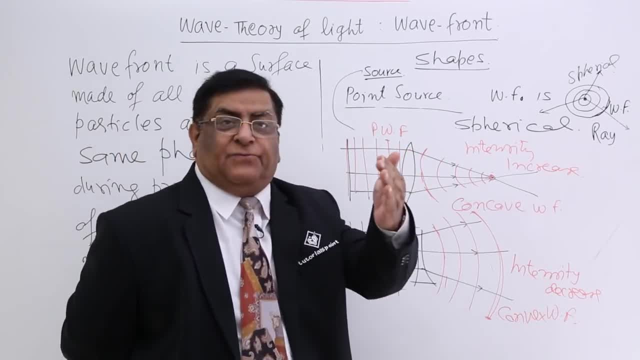 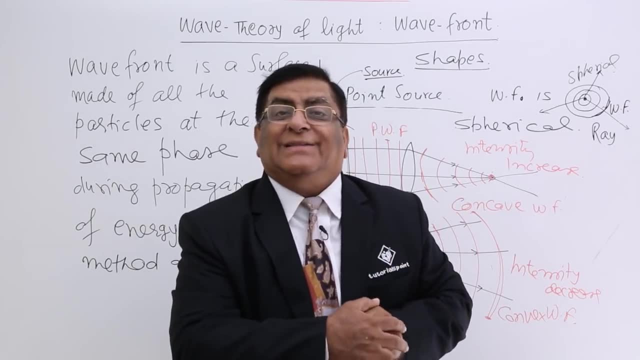 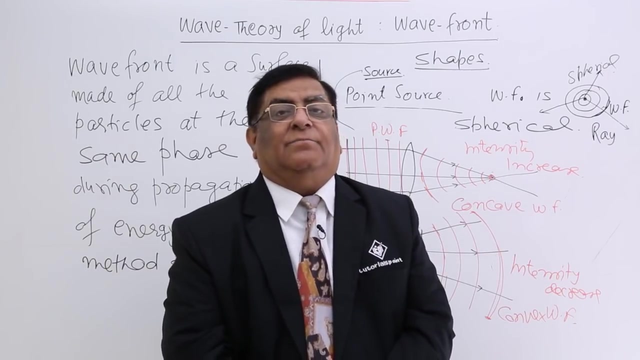 Because of the source of light, one wave front is formed, Then there is another wave front is formed, Then third wave front is formed. There is a mechanics How a new wave front is formed. A little bit difficult to think, that if there is a disturbance and one wave front is formed.